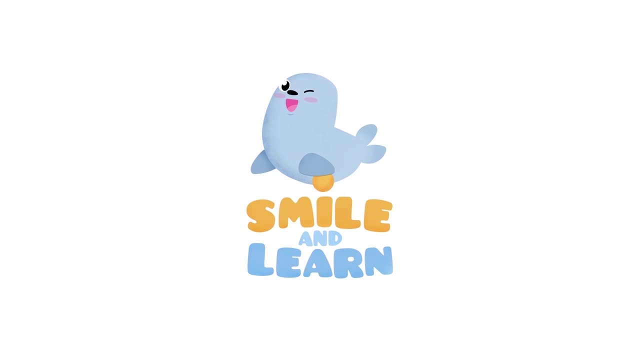 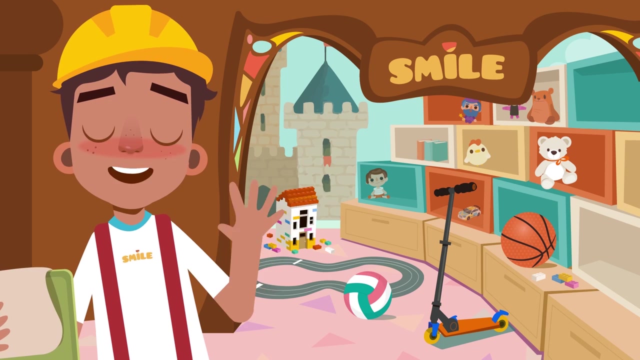 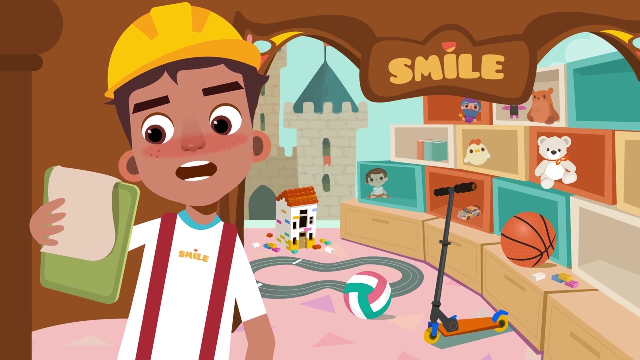 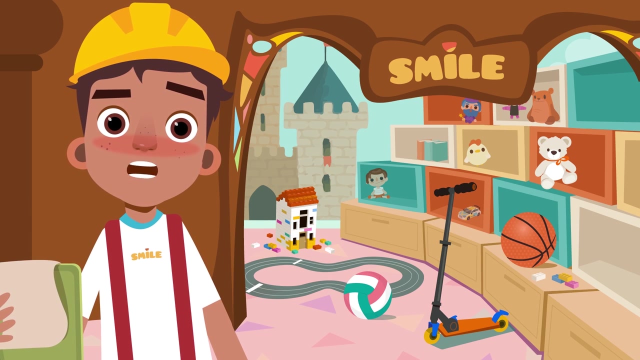 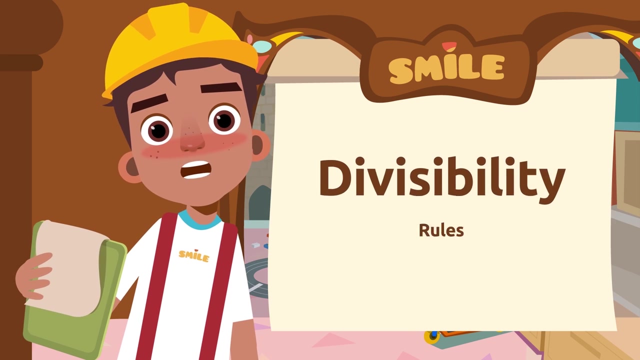 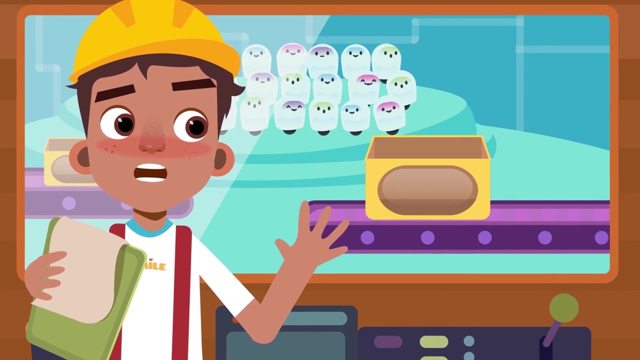 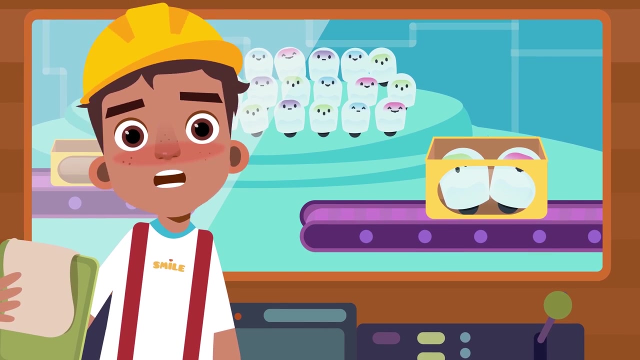 Smile and Learn. We call them the divisibility rules. I'll tell you about some of them. Look at how many robots there are. We want to put two in each box, but we need to know if there will be any left over. We can't send any boxes with only one robot. 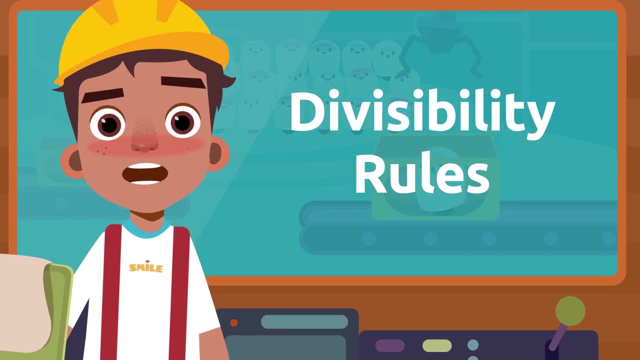 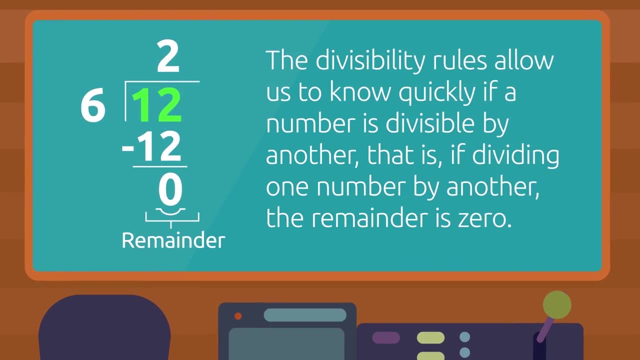 To find out, we'll be using the divisibility rules. The divisibility rules allow us to know quickly if a number is divisible by another, that is, if a number is divisible by a number, That is, if, dividing one number by another, the remainder is zero. 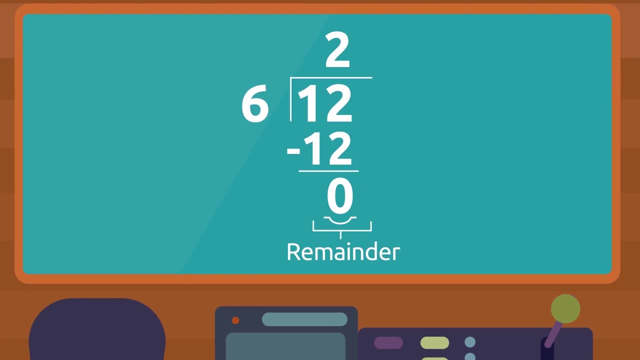 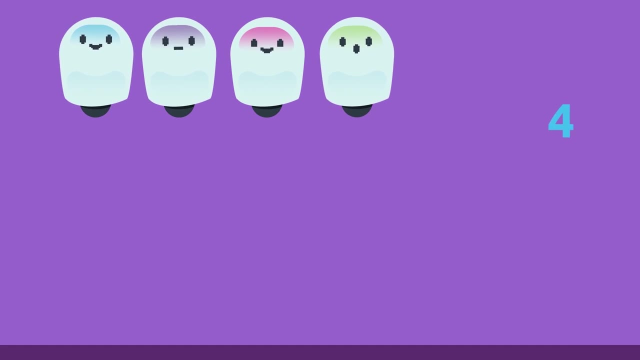 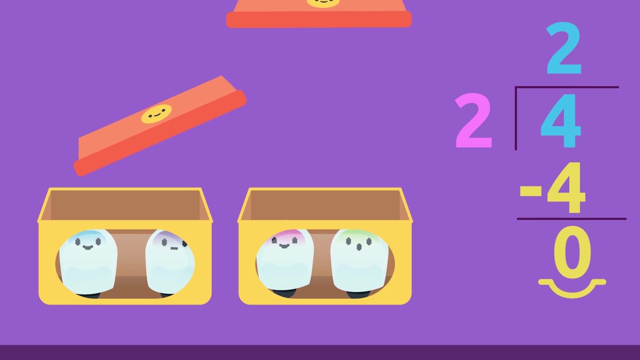 When a number is divisible by another number, the number that we have divided it by is called the divisor. For example, if we have four robots and we want to put two in each box, there won't be any left over because the remainder of the division is zero. So four is divisible by two, and the number 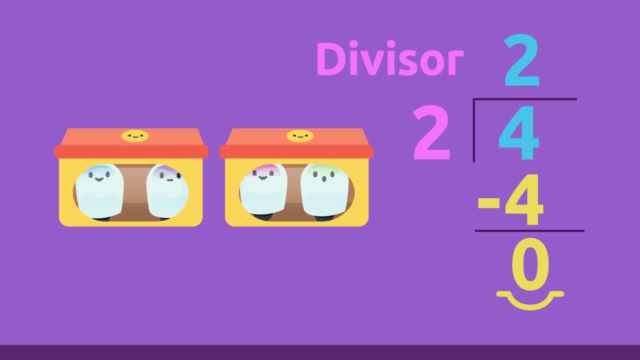 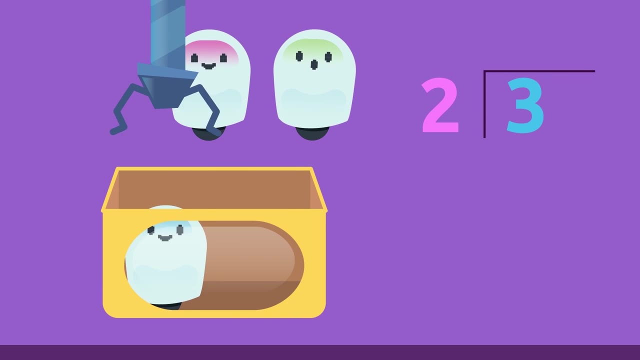 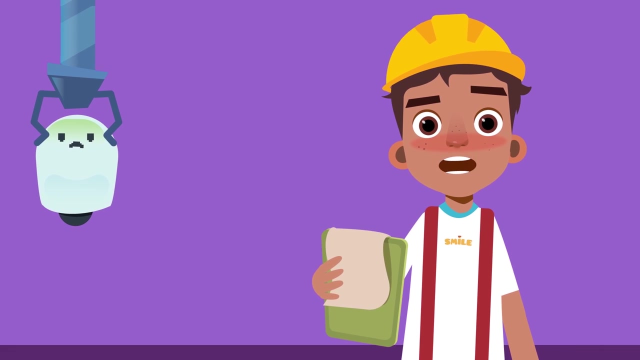 two is its divisor. For example, the number three isn't divisible by two because if we divide three by two, the remainder isn't zero. Look, the remainder is one. Each number has its own divisibility rule. Some are based on adding all the digits. 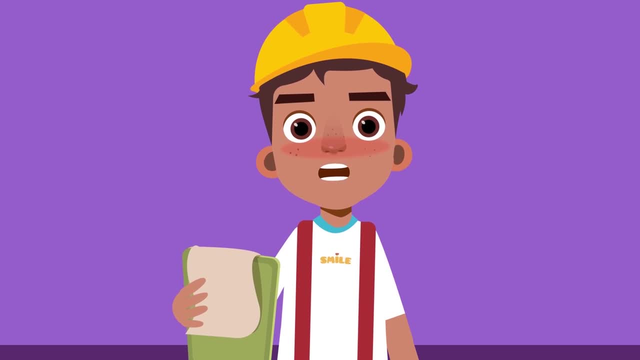 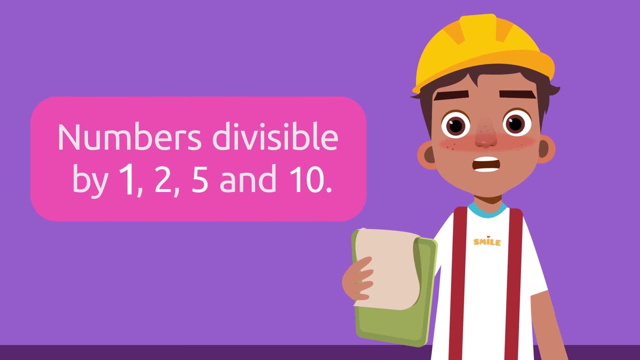 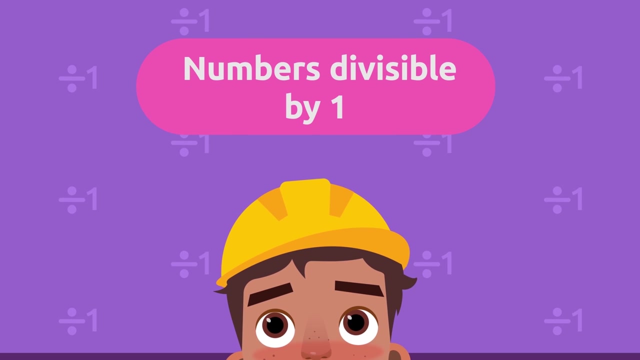 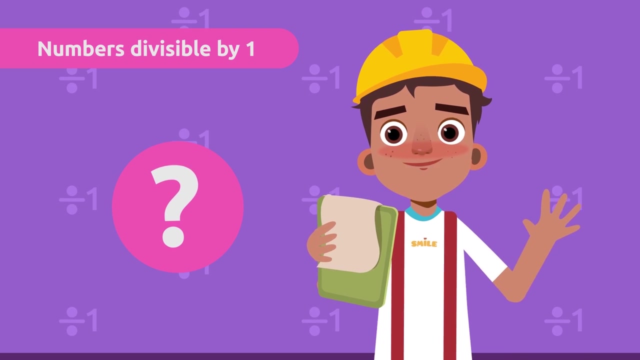 For others, you have to look at the last digits and say some can be done by doing several simple operations. Today we'll talk about the numbers divisible by one, two, five and ten Numbers divisible by one. There's a very special number which no divisibility rule is needed, because any 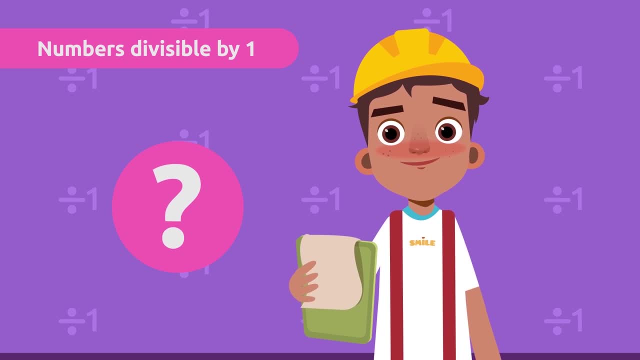 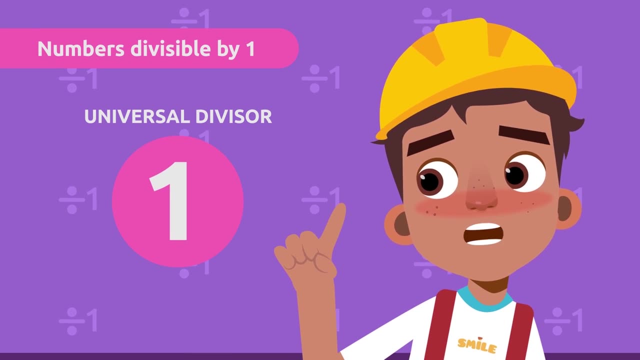 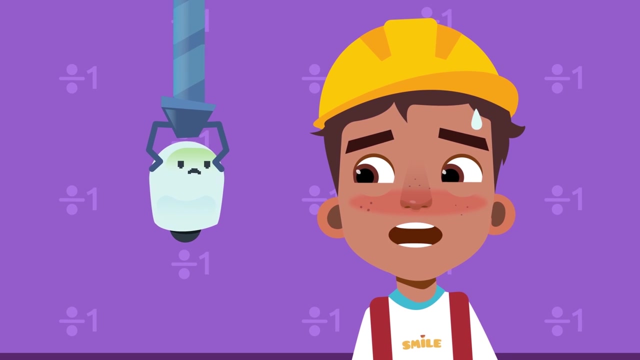 number you can think of is divisible by it. It's known as the universal divisor. Can you tell me what? it is Correct? The number one, Every number, can be divided by one and the remainder will always be zero. All right, let's go solve our robot problem. 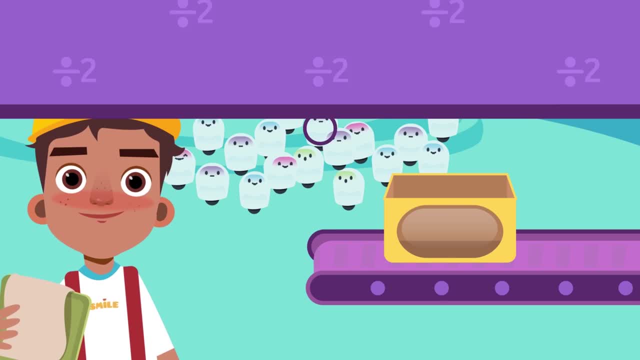 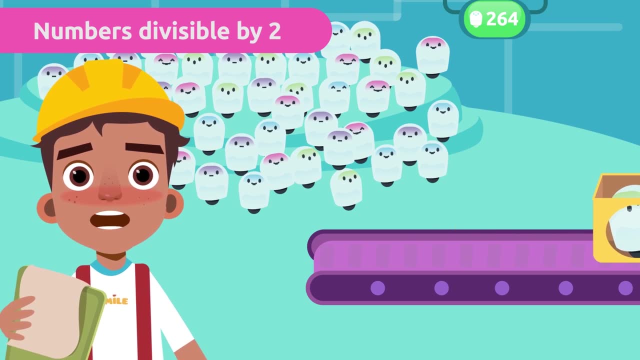 Numbers divisible by two. As you see, there are 264 robots and, as I told you before that I'd want to divide them by two, I'd want to put two robots in each box. We need to know if all the boxes will be. 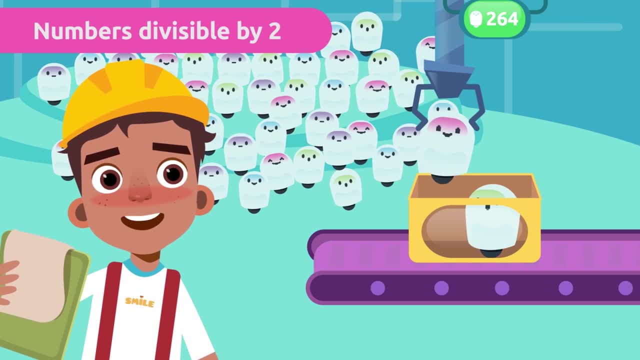 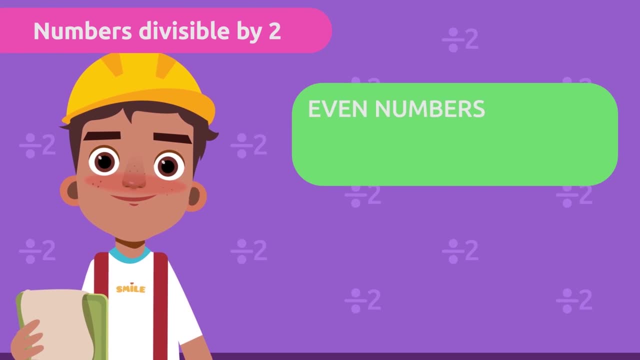 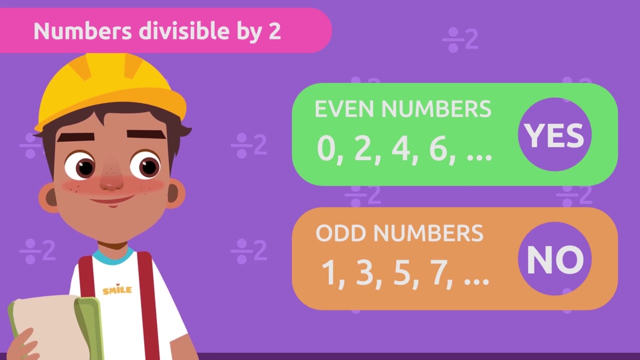 full or if there will be robots left over. It's very easy to figure out. We can use the divisibility rule of two. If it's an even number, it's divisible by two, and if it's an odd number, it isn't divisible by two. The remainder is one which is: 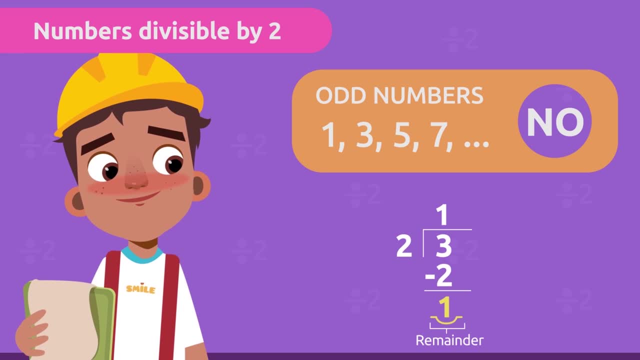 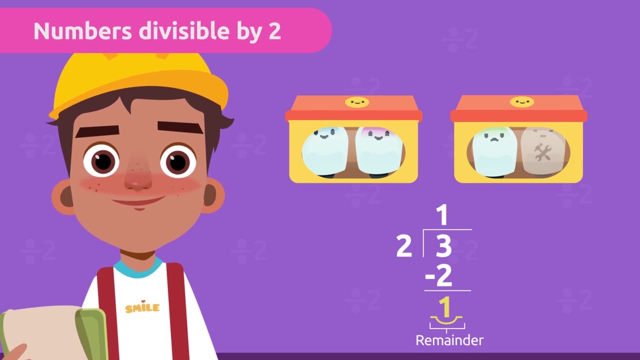 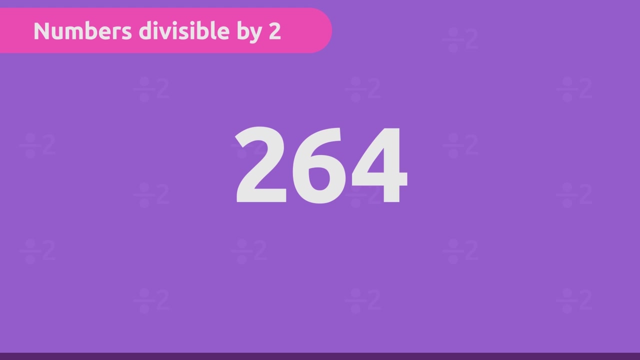 the number of robots left over. That means we will have one robot left over and we would have to make one more to fill the box. Let's give it a try To figure out if a number is odd, or even we have to look at its last digit. The last digit of 264 is four which. 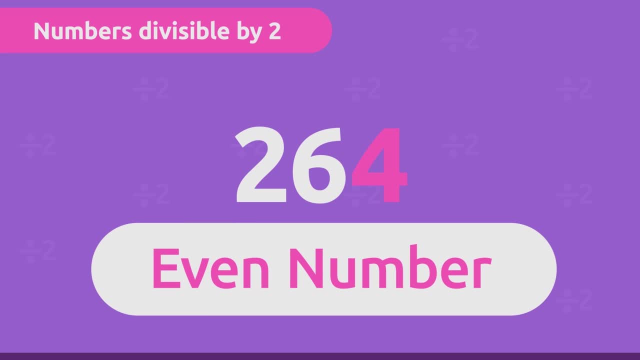 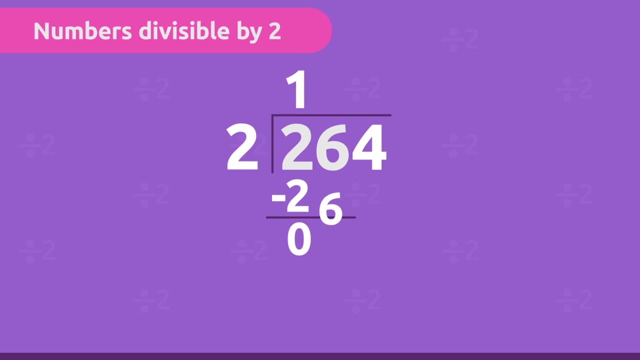 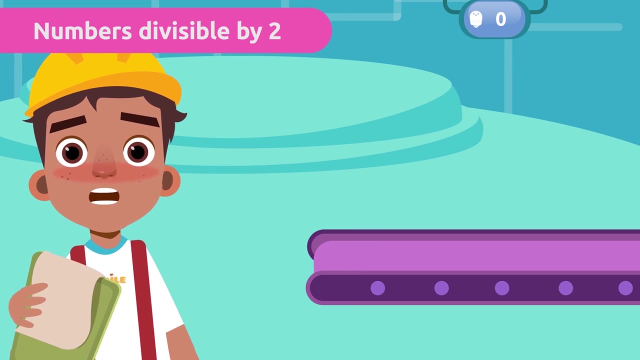 is an even number, So 264 is even and it should be divisible by two. Let's test the robot. Here's the divisibility rule. Look, The remainder is zero and we have proven that the divisibility rule of two works. Fantastic, No robot was left over. 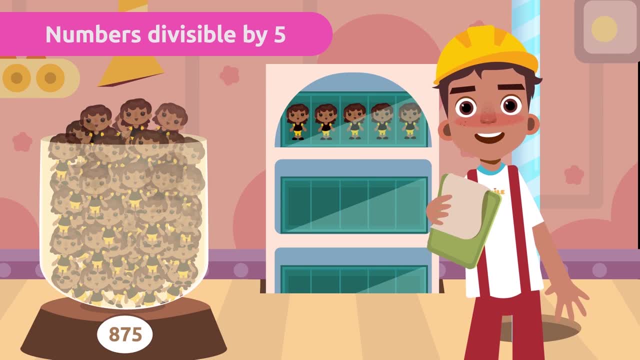 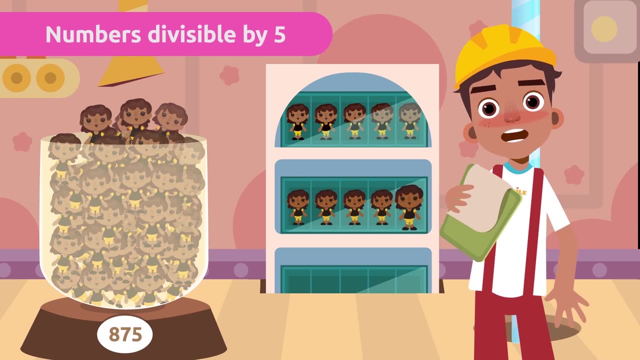 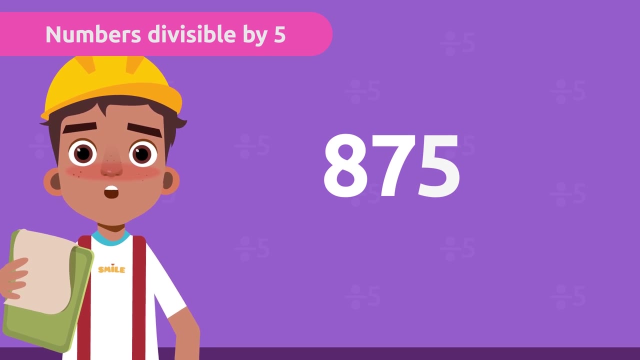 Numbers divisible by five. Here we have dolls In this case. we can always keep five in each box To find out if we can divide them into boxes of five. we use the divisibility rule of five To find out if a whole number is divisible by five. we only have to look at the last. 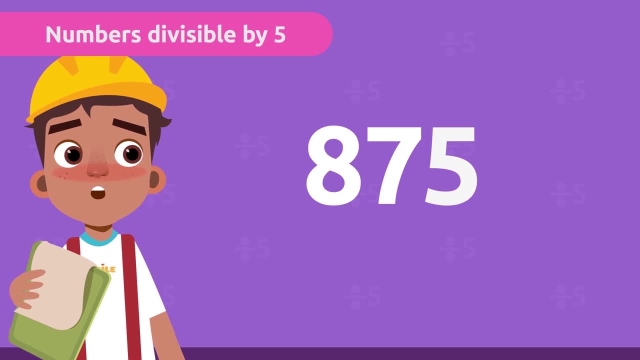 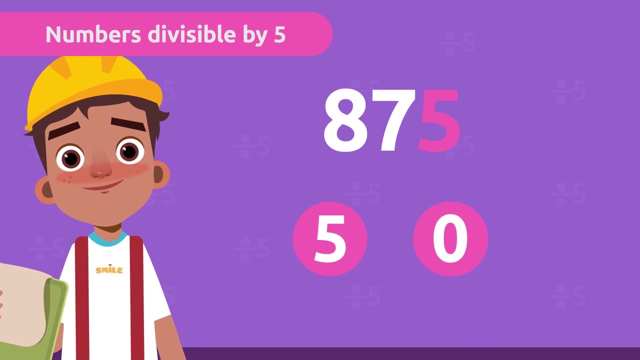 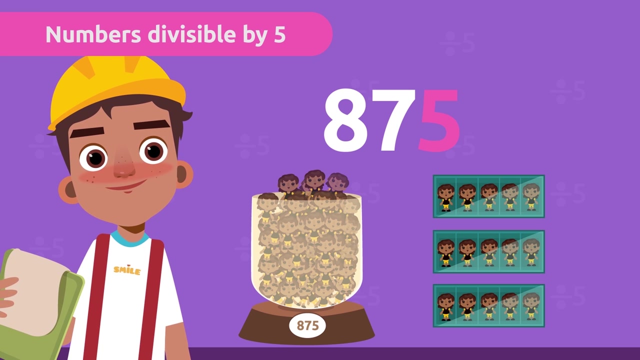 digit. It's super easy. Every number ending in five or zero is divisible by five. There are 875 dolls, so if we store them five by five, there will be none left over. You know why? Think of the multiplication table of five. 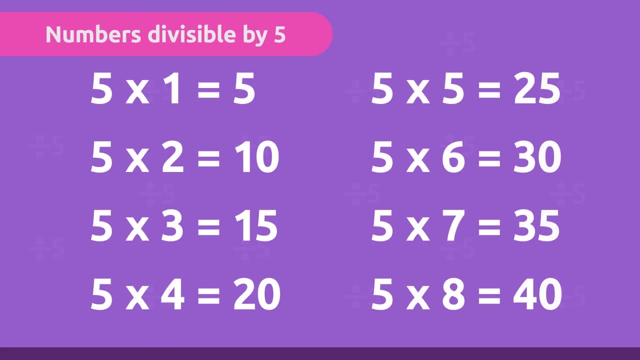 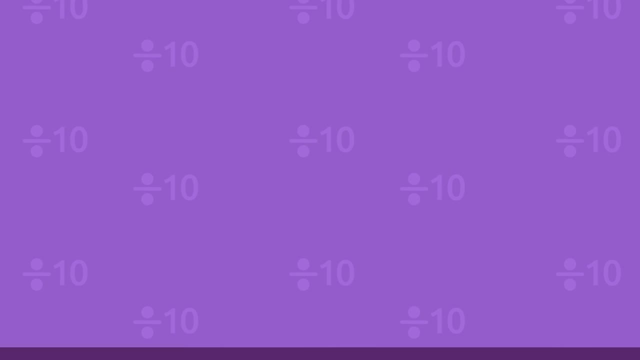 Let's look at the last digits. Did you notice anything Exactly? All the results end in five and zero, as in our divisibility rule of five. Let's go to the marble area Numbers divisible by 10.. Let's go to the marble area Numbers divisible by ten. 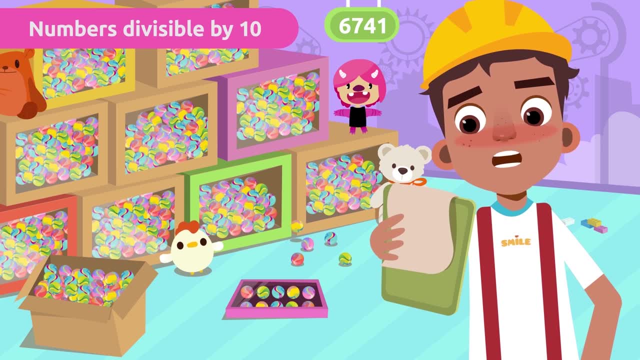 Numbers divisible by seven. Numbers divisible by eight. Numbers divisible by nine. Numbers divisible by twenty. Numbers divisible by ten. Numbers divisible by sixty. Numbers divisible by 6741 marbles, we're putting 10 in each box. now we need to know the divisibility rule for the 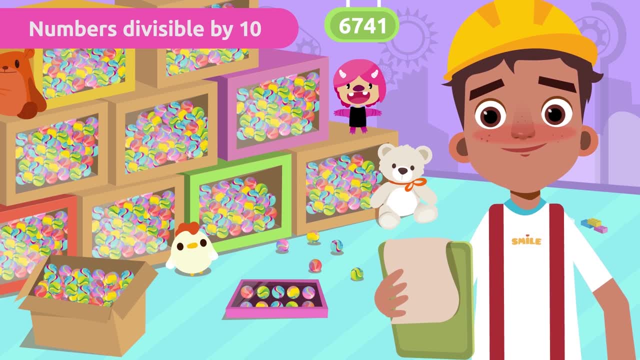 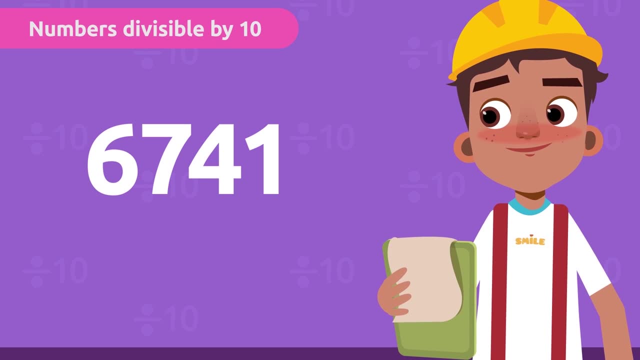 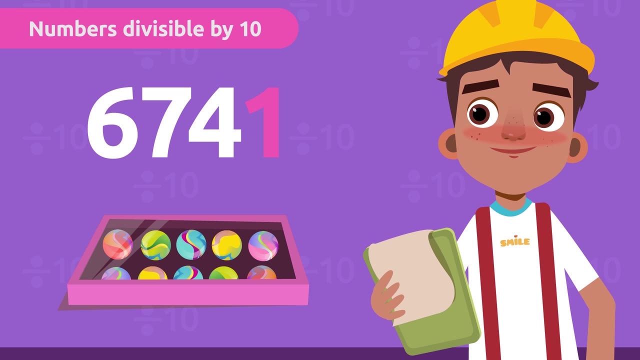 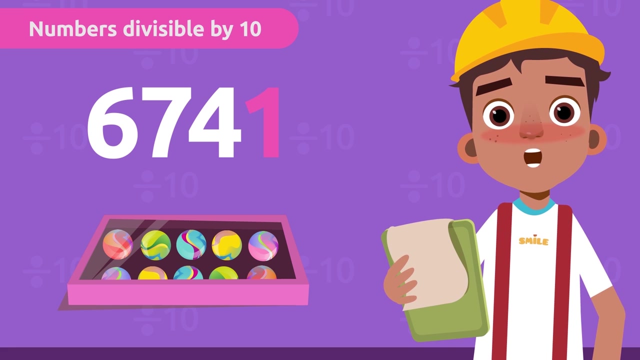 number 10 so that there are no marbles left over. this is much easier. we just have to check. if the number we want to divide ends in zero, what do you think will happen when we pack up all our marbles? very good, there will be marbles left over because the number 6741 is not divisible by 10, can you? 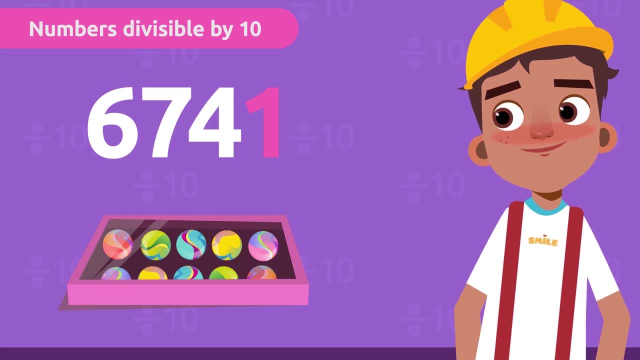 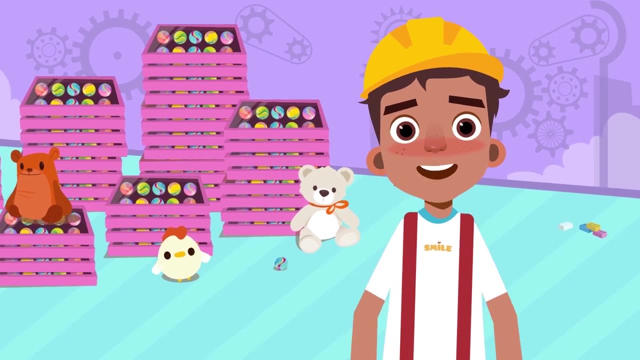 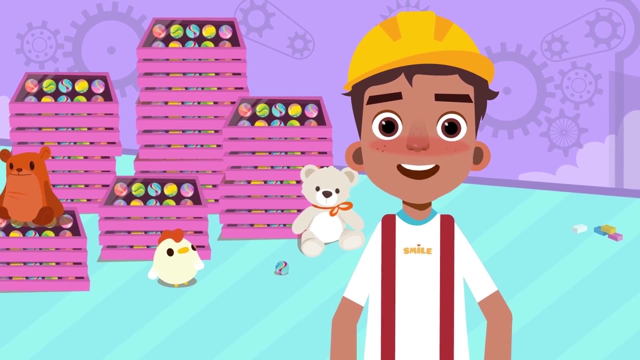 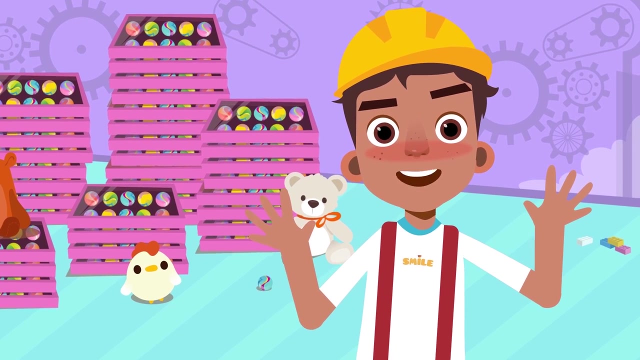 guess how many we will have left over. there will be one left over. well done. thank you very much for your visit. I hope you enjoyed learning about the divisibility rules. they are very useful in everyday life. they will also be useful in your math classes at school because they give us clues to simplify fractions, to know if a number is prime and a lot. 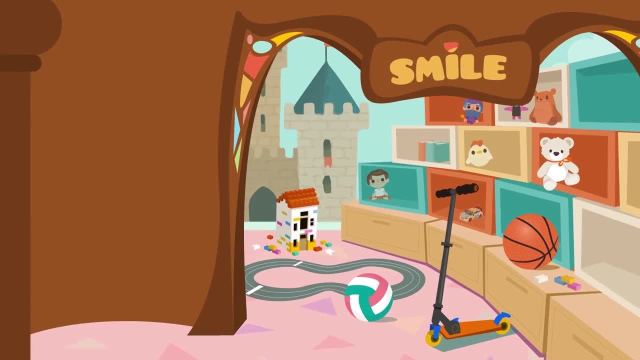 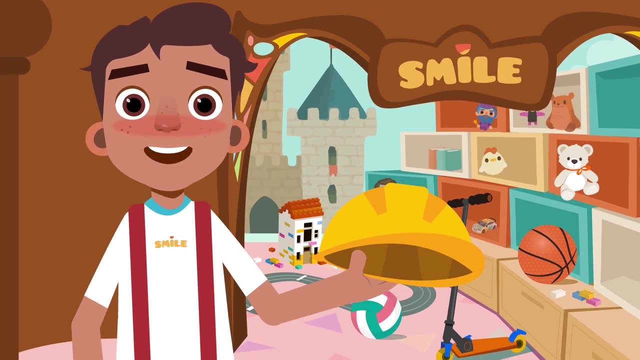 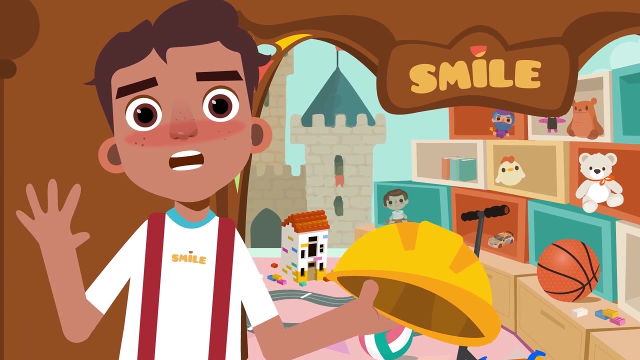 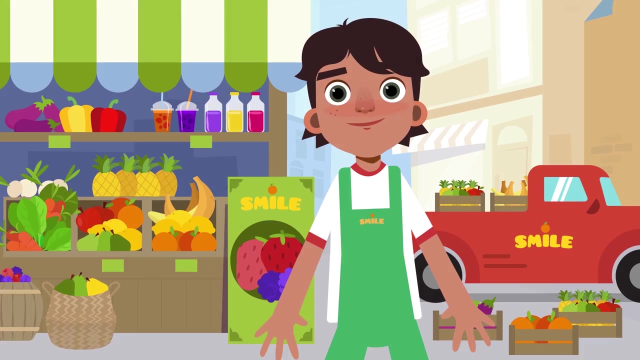 of other things, time for a break. if you're hungry, you can stop by my brother Connor's fruit shop. he's right next door and he loves to be visited so he can teach his favorite divisibility rules. you'll have a great time. see you later, hello. welcome to smile fruit shop, where you can find the best fruit on the market. 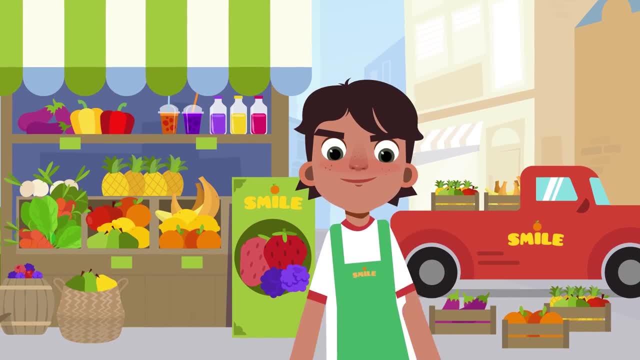 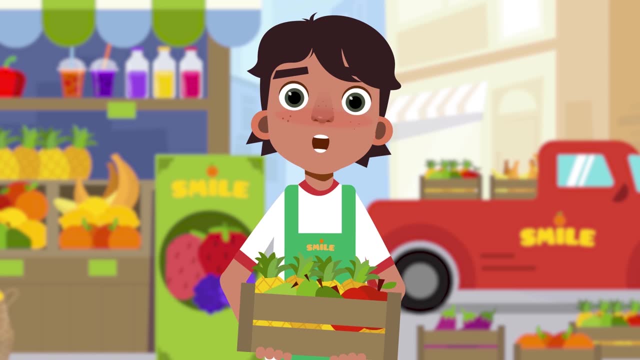 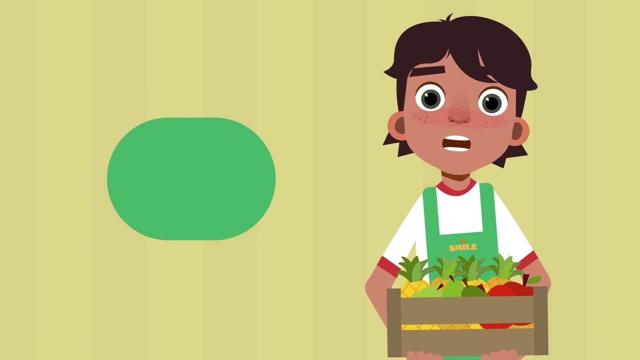 my name is Connor divisor, nice to meet you. I'm preparing boxes fruit to send to the neighborhood soup kitchen to find out if I have any pieces of fruit left over when I put them in boxes. I will use the same trick. my brother, Windsor divisor, uses the divisibility rules. 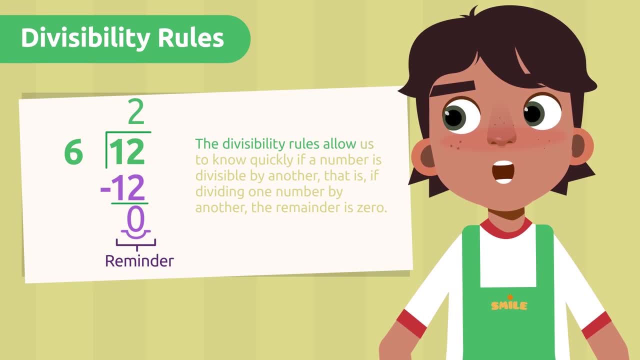 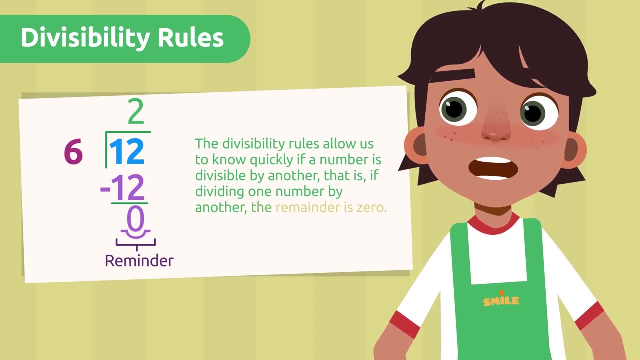 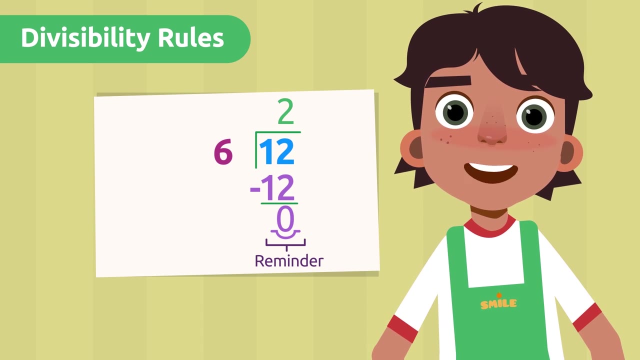 the divisibility rules are the same as the divisibility rules are the same as the divisibility rules allow us to know quickly if a number is divisible by another, that is, if, dividing one number by another, the remainder is zero. when a number is divisible by another number, the number 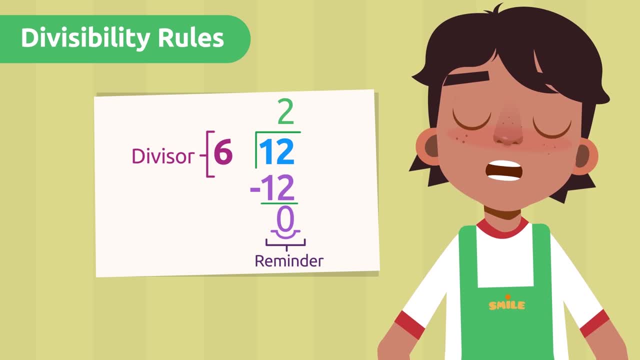 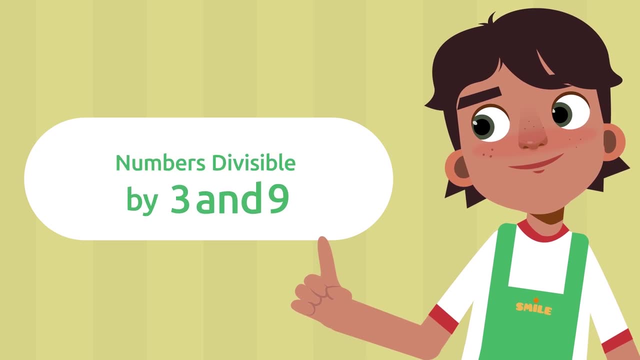 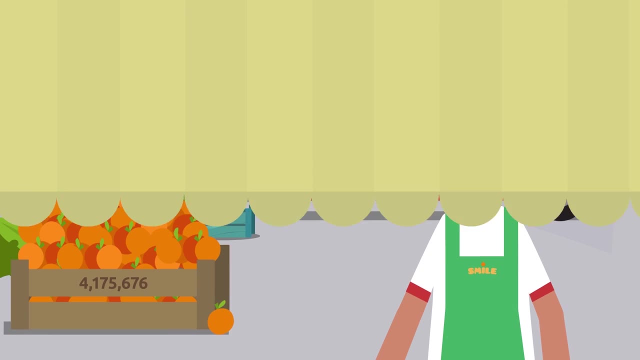 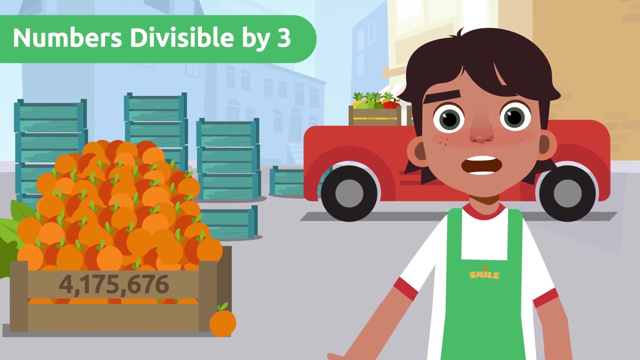 that we have divided it by is known to be its divisor. today, we'll talk about all those numbers that are divisible by three and nine numbers divisible by three and nine divisible by three. I want to put three oranges in each box to find out if the number can be divided by three. there's. 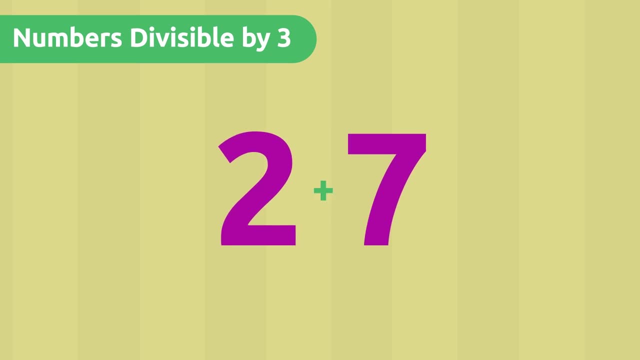 a neat trick. we have to add up all the digits and if the result is divisible by three, then the original number is two. let's see what happens with all the oranges we have. there are four million one hundred and seventy-five thousand six hundred and seventy-six oranges. 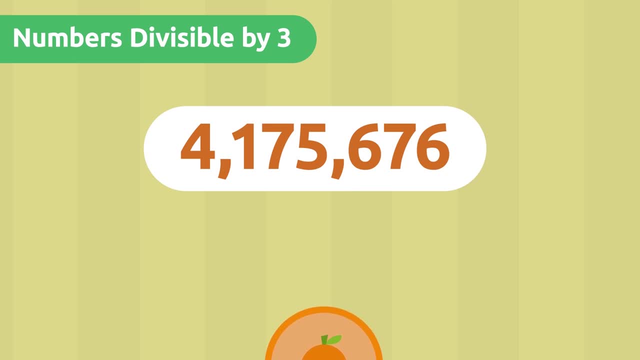 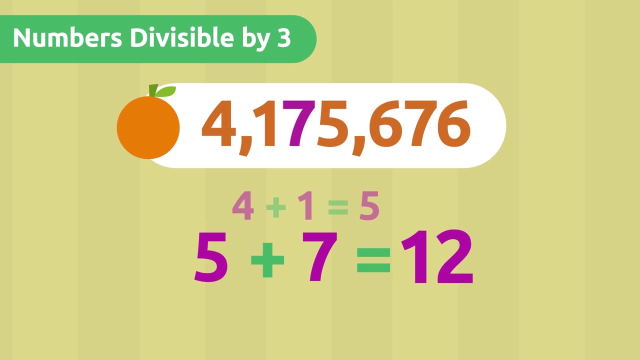 to sort. that's a huge number, but that's okay, we'll do it one step at a time. four plus one is five. five plus seven is twelve. twelve plus five is seventeen. seventeen plus six is twenty-three. twenty-three plus seven is thirty, and thirty plus six is thirty-six. let's check if thirty-six is divisible by three. 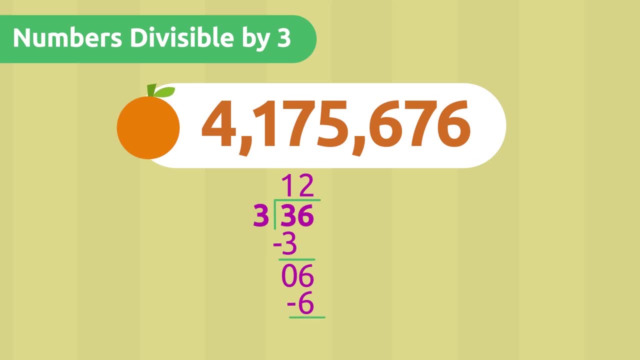 in this case, dividing thirty-six by three, the remainder is zero. that means thirty-six is divisible by three. since thirty-six is the result of adding the oranges, applying the divisibility rule of three means that there will be none left over if we pack three in each box. 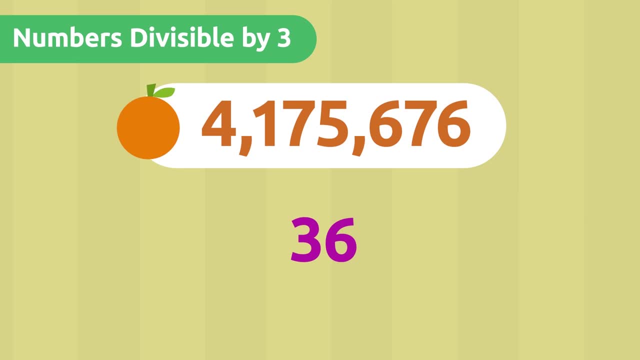 but what happens if we add the digits of a number and we get a very huge number? doing division with such a large number would take us a long time and what we want to know quickly is the divisibility of a number in that case, after adding up the digits of the original. 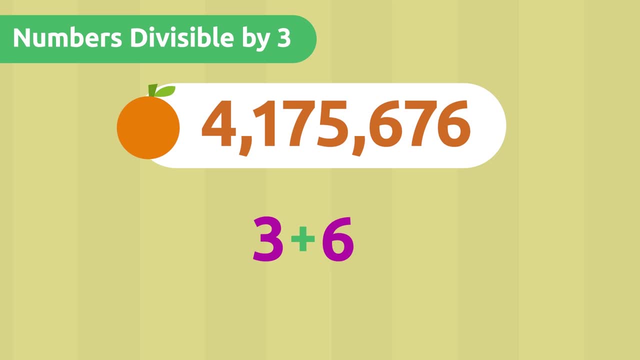 number, we would go back and add again the digits of that number which we have obtained as a result to get a smaller number. if we get a number divisible by three, then the original number should also be divisible by three. when we added the number of oranges, we got thirty-six. if we add up the digits of thirty-six, 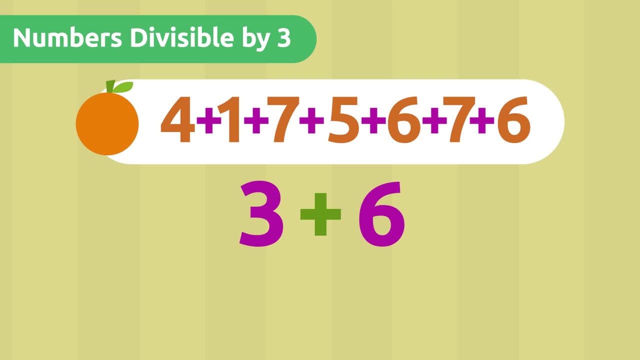 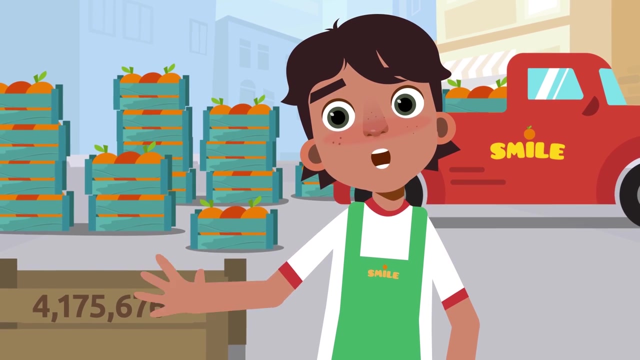 we should have a number divisible by three. let's test our theory by adding its digits. nine is a very small number and we know that if we divide it by three, the remainder will be zero. the divisibility rule of three is super fun because we can add digits as many times as 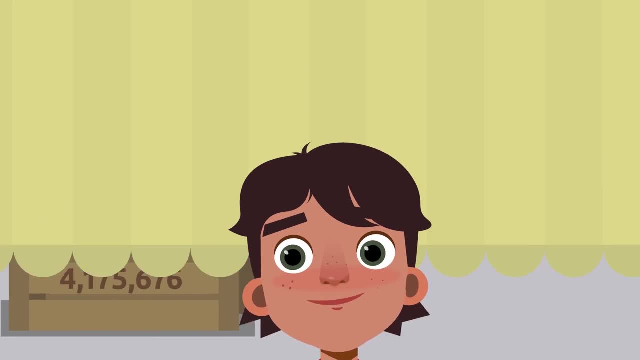 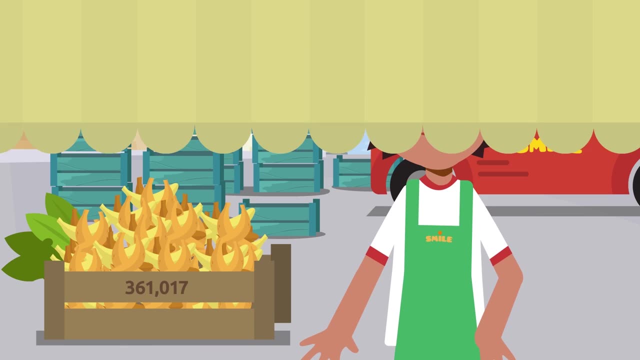 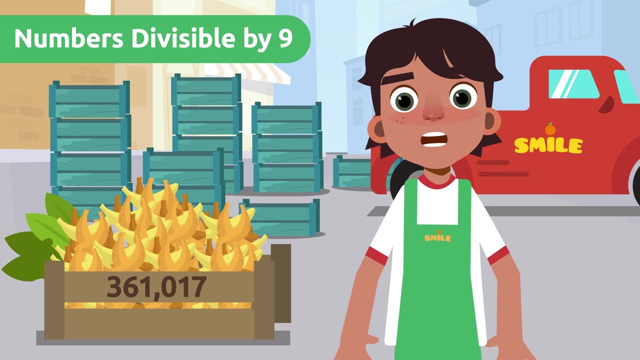 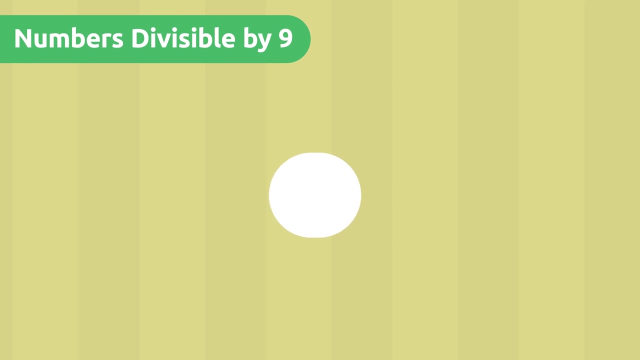 we need- isn't it very useful? numbers divisible by nine. we also send bananas. they are very healthy. there are three hundred and sixty one thousand and seventeen bananas and we'll send nine per box. let's see if we have any leftover. the divisibility rule of nine: 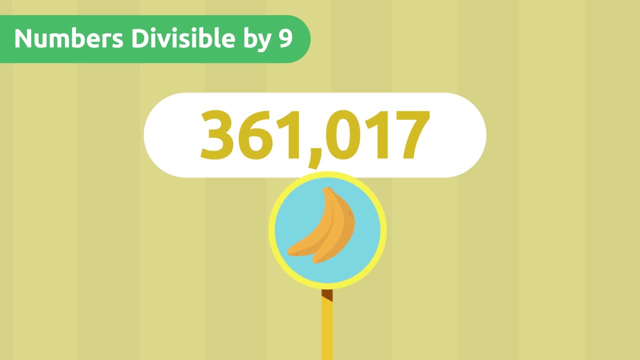 is calculated in the same way as the number three. we have to add it's digits, divide the result by nine and check that the remainder is 0. take a look: 3 plus 6 is 9, 9 plus 1 is 10, 10 plus 1 is 11. 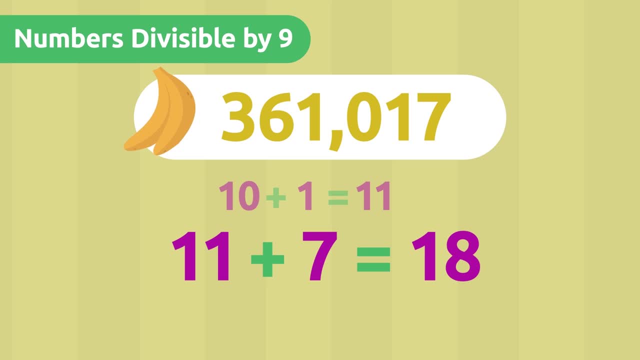 And 11 plus 7 is 18.. Now we'll do the division, Since the remainder is 0,, 18 is divisible by 9, and so is the number of bananas. That means we won't have any bananas left over when we put them in the boxes. 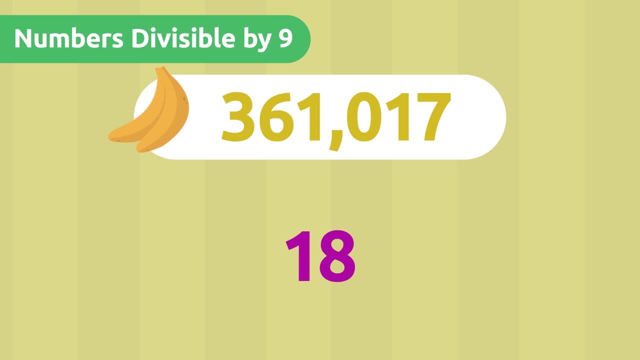 But, as with the divisibility rule of 3,, the result of the sum of the number we want to check may be too large of a number. What do you think we could do then? Exactly, We are going to do the same as before, so we need to add their numbers again. 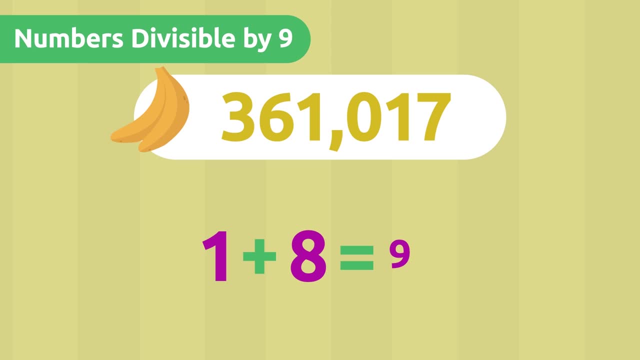 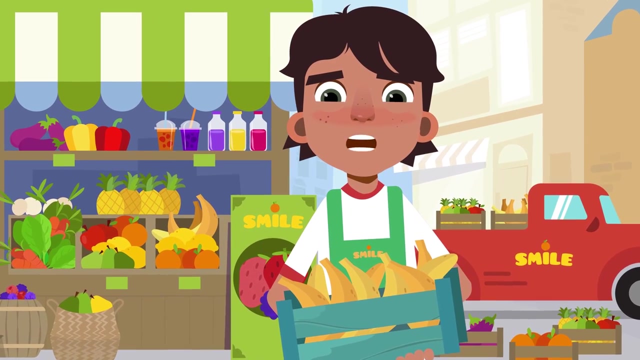 The previous sum gave us 18. So 1 plus 8 is 9.. A number is always divisible by itself, so we have already solved the banana problem. Whew, I'll be here for a long time loading these boxes. You can walk around. 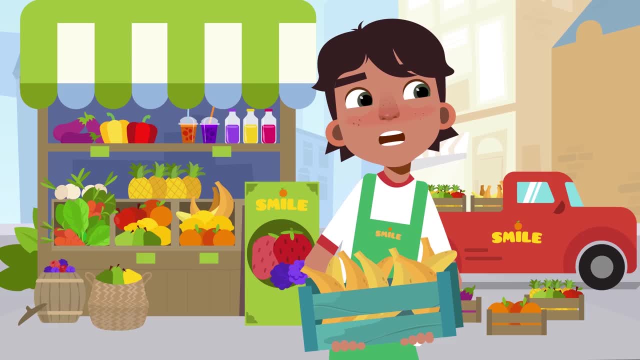 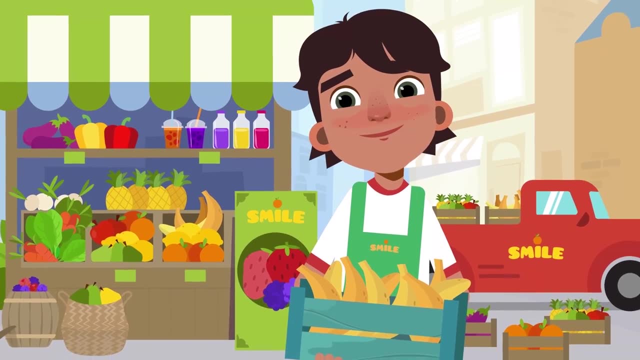 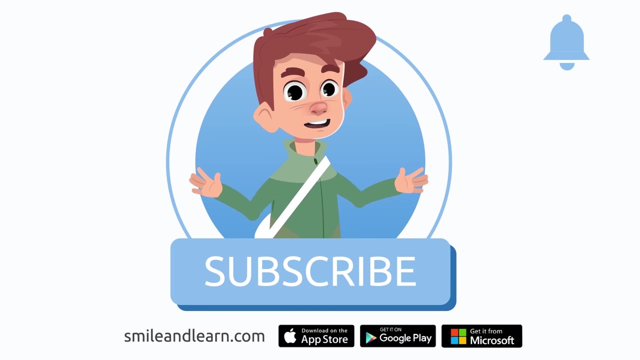 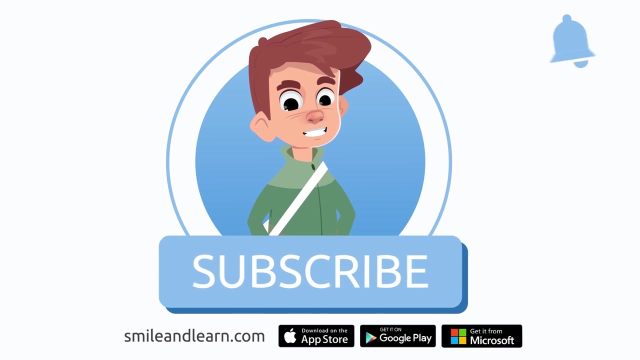 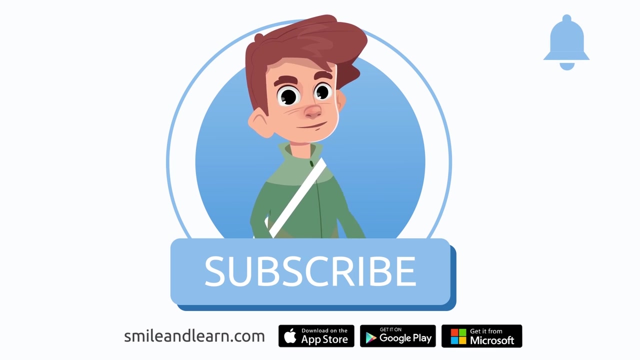 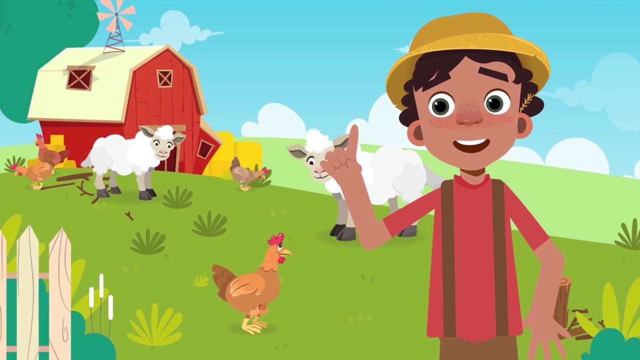 In the meantime, why don't you visit my brother Trevor's organic farm? I'm sure he could explain some divisibility rules. you don't know yet. See you soon. Good morning. welcome to my little farm. my name is Trevor Divisor. I'm super excited. 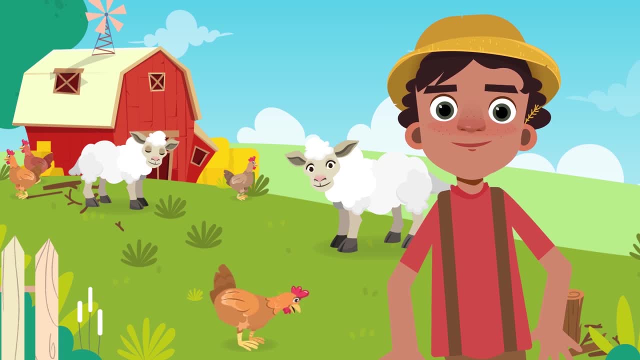 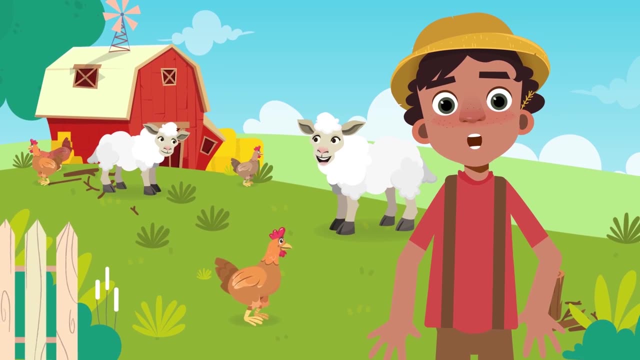 for your visit. I have a lot of animals, mostly sheep and chickens. You can see that they have plenty of room to roam, but now that winter is coming they will need shelter. I want my animals to be very comfortable, so I will build stables and chicken coops. 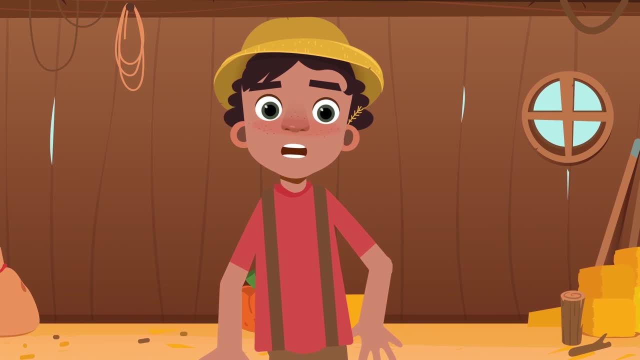 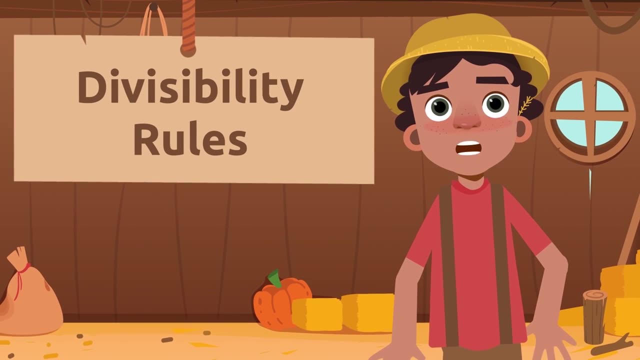 where I will group them. It's important that the chicken coops and stables are full and that there aren't any of them left out in the cold. For that I will use the divisibility rule. It's a custom in my family. 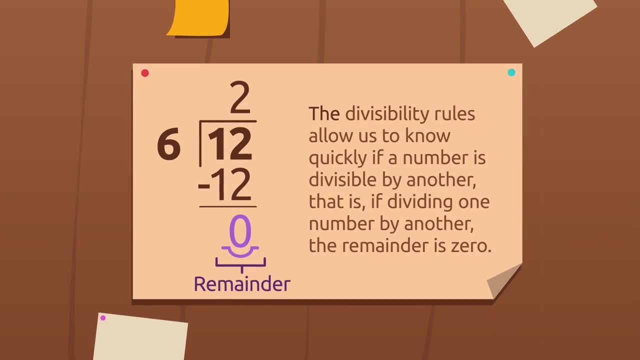 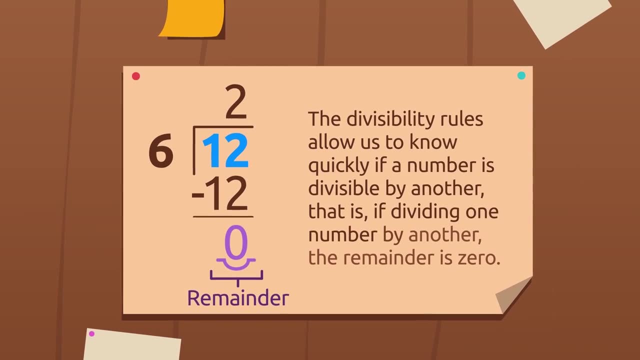 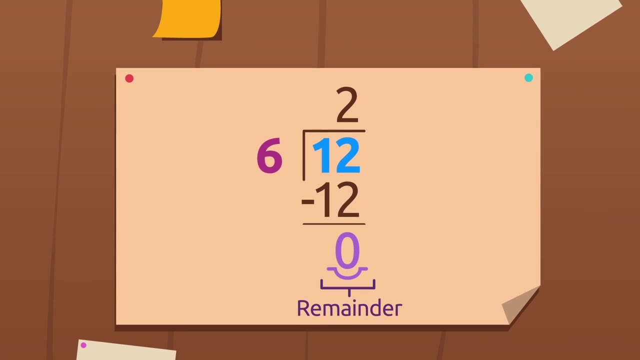 Do you want me to remind you? The divisibility rules allow us to know quickly if a number is divisible by another, That is, if, dividing one number by another, the remainder is zero. When a number is divisible by another number, the number that we have divided it by is a. 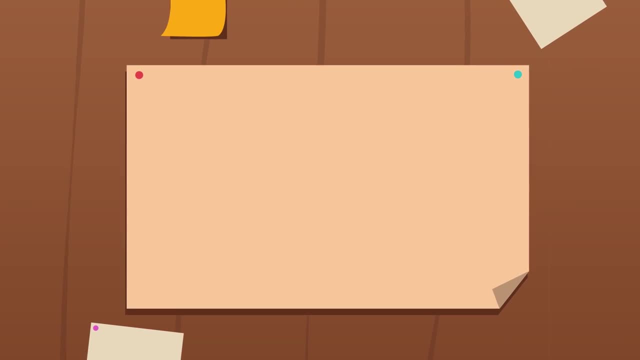 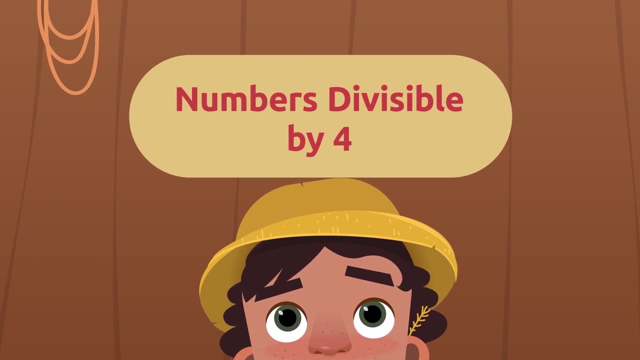 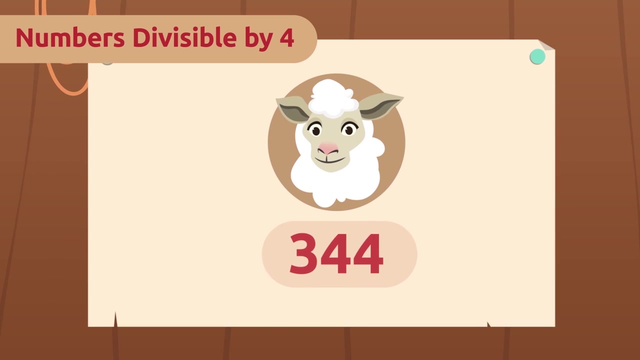 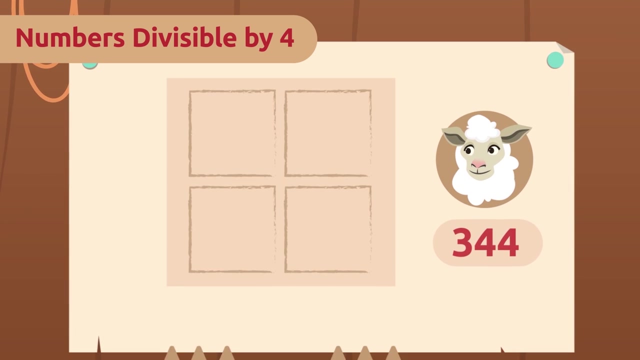 divisor. Today we will learn about the numbers that are divisible by 4 and 8.. Numbers Divisible by 4. I love my sheep very much. I know all 344 names. As I want them to be comfortable, I have thought about building stables where they can rest. 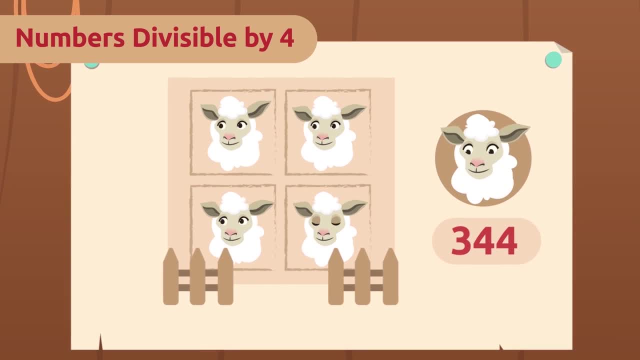 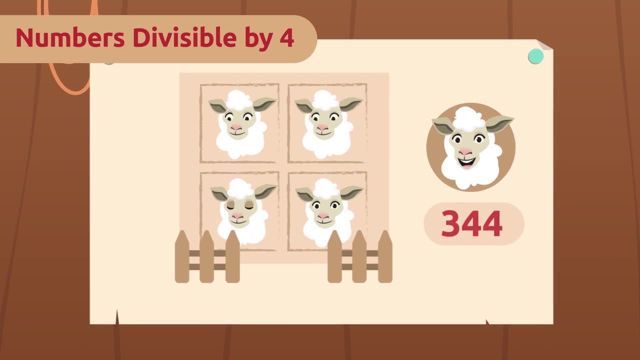 in groups of 4 without any of them being left out. Let's get started. Let's recap: There are 344 sheep and I want 4 to sleep in each stable. To find out if I can put them in groups of 4 without any left in the cold, I will use. 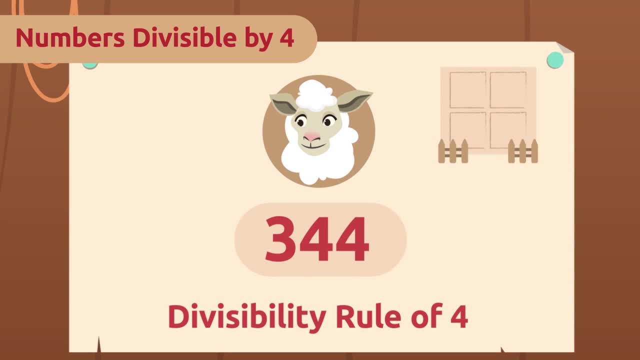 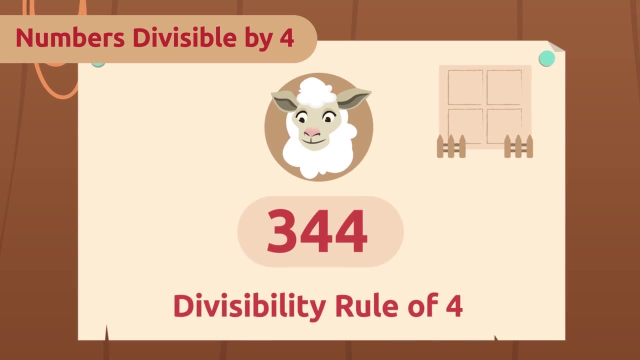 the divisibility rule of 4.. The method is based on two rules. If any of them is fulfilled, it means that our number is divisible by 4.. First, we have to check if the last two digits of the number we want to divide are zeros. 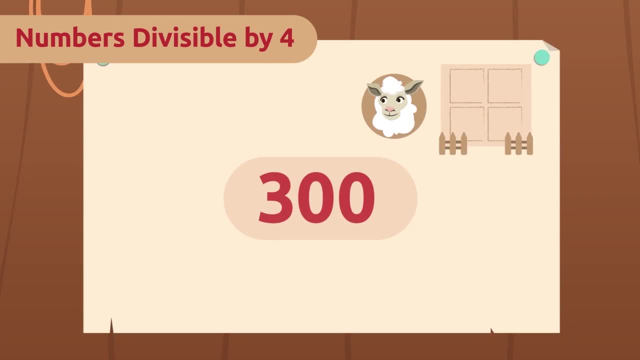 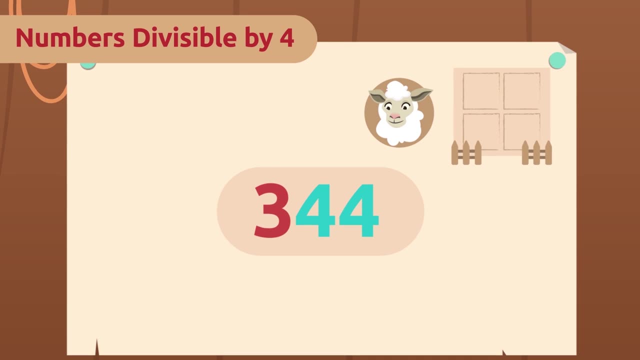 If so, then we already know that it is a divisible number. We already know that it is divisible by 4.. Let's check the number of sheep I have. Wow, it is 344!. The number doesn't end in two zeros, so we have to check its divisibility with the other. 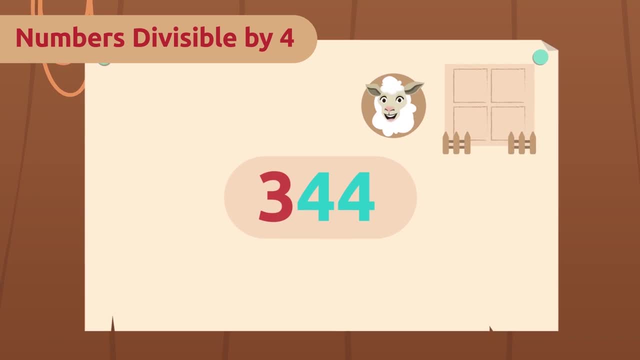 rule I was telling you about. We will continue to look at the last two digits, but this time we will check if the number they form is divisible by 4.. There are 344 sheep, so the last two digits are 44. Let's try dividing 44 by 4.. 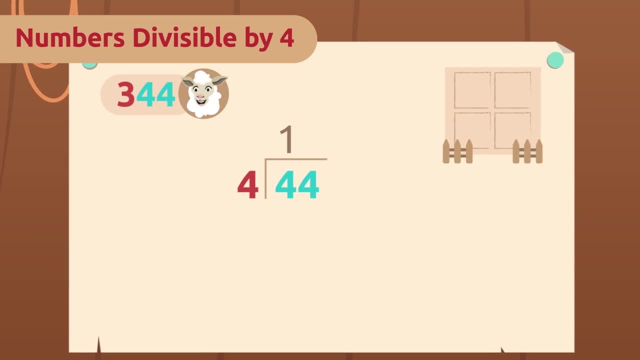 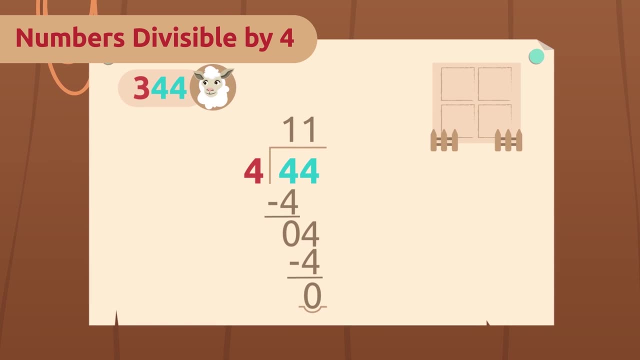 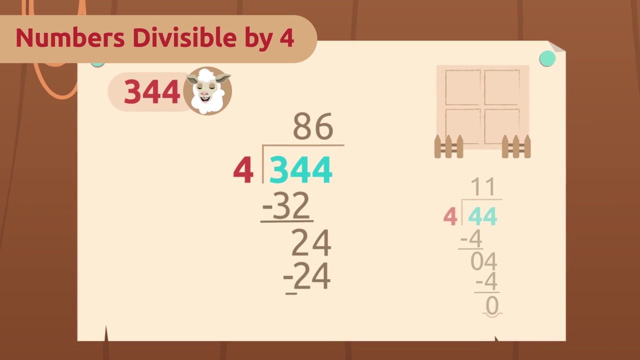 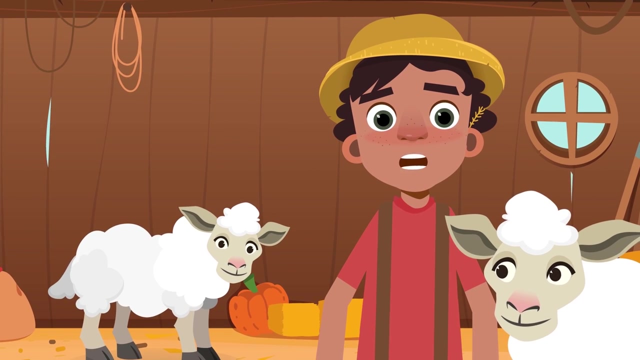 dividing 44 by 4 and see if the remainder is 0.. Yes, the remainder is 0,, which means that our original number, 344, is also divisible by 4.. Awesome, All the stables will be full. I'll have to work hard before winter comes. I don't want my 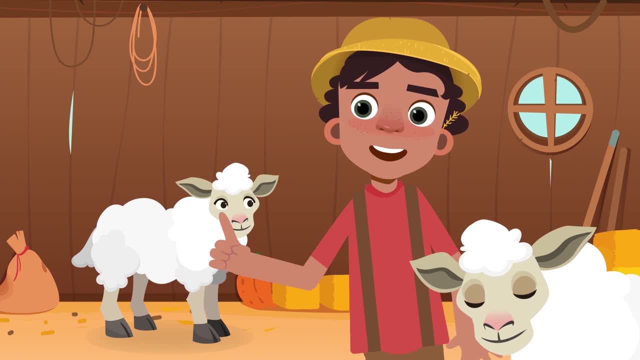 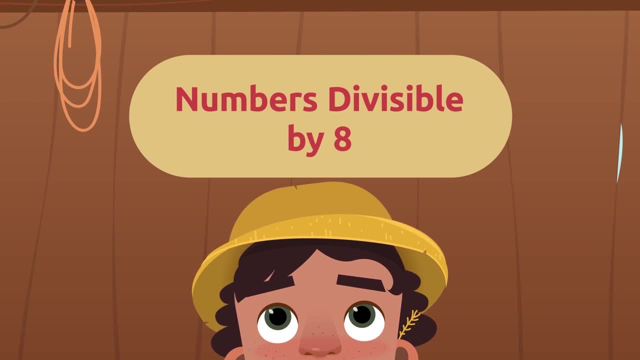 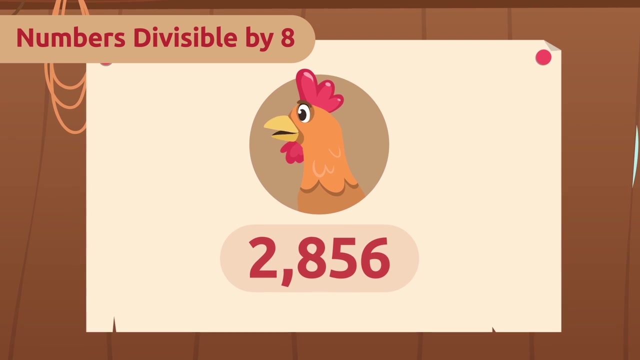 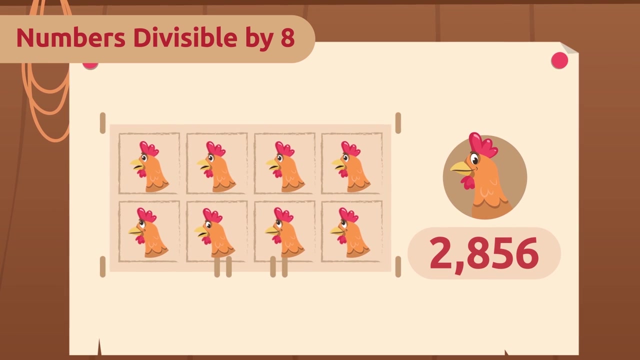 wooly friends to be cold. Come on, let's go to the chicken area now. Numbers divisible by 8.. There are 2,856 hens and, believe it or not, I know all of their names too. I'm going to build 8 cedar coops. It's the perfect number for them. 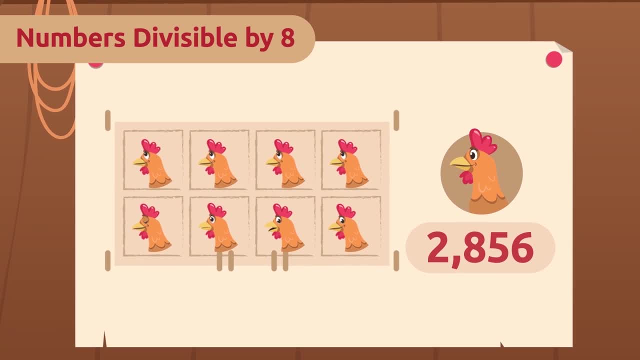 to be comfortable. but I have the same question as before: Will any chicken coop be comfortable? I'm going to build 8 cedar coops. It's the perfect number for them to be comfortable. but I have the same question as before: Will any chicken coop be? 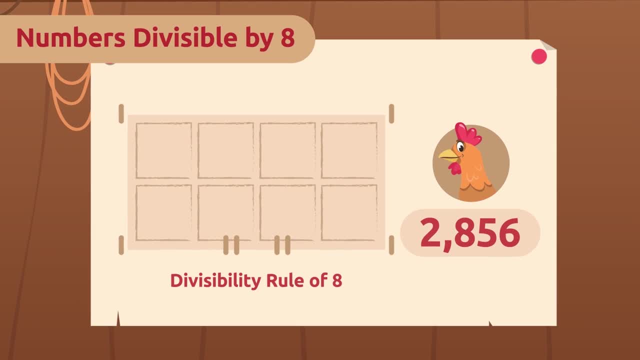 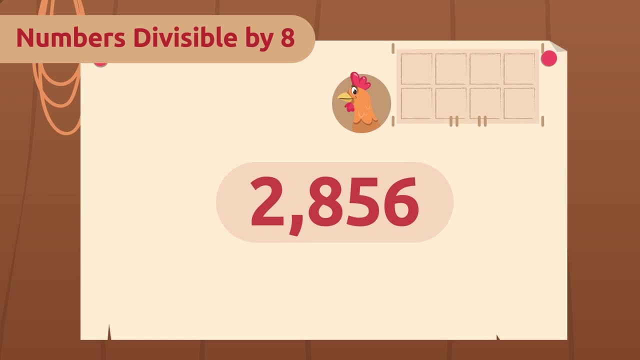 incomplete. To get rid of any doubt, I will use the divisibility rule of 8.. With such a large number, it will be very useful. Let's go To find out which numbers are divisible by 8,. we have to look at their last three digits and see if they. 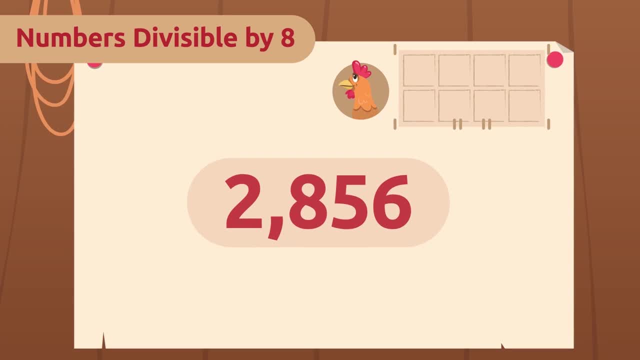 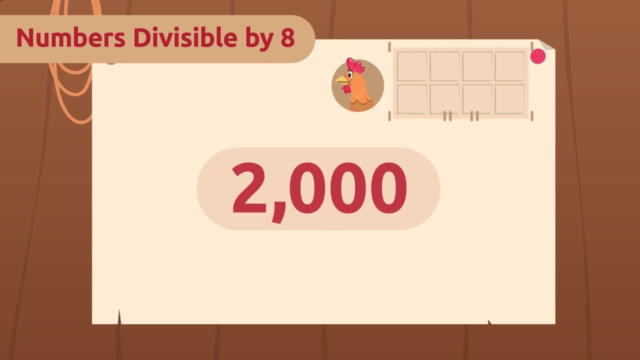 meet one of the two criterias for the divisibility rule of 8.. First we will check if the last three digits are three zeros. The last three digits of our number are 8,, 5,, 6,, so this criteria is: 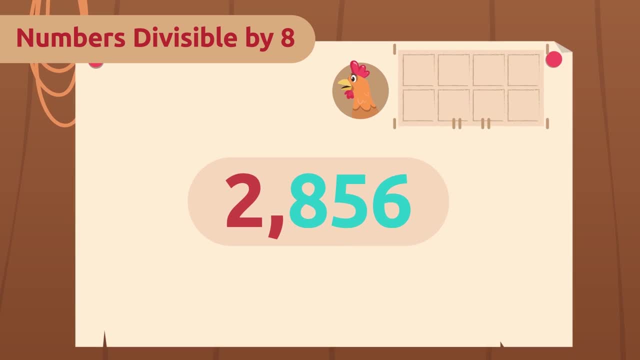 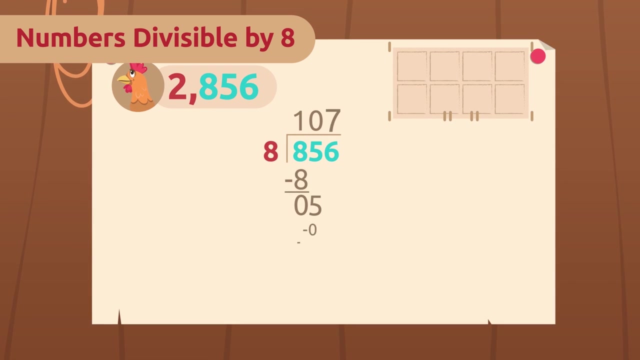 not met. Oh man, Second rule: we will check if the last three numbers are divisible by 8.. That is, we have to divide them by 8 and look at the remainder. Let's do it. The remainder of 856 divided by 8 is 0. That is, it is a. 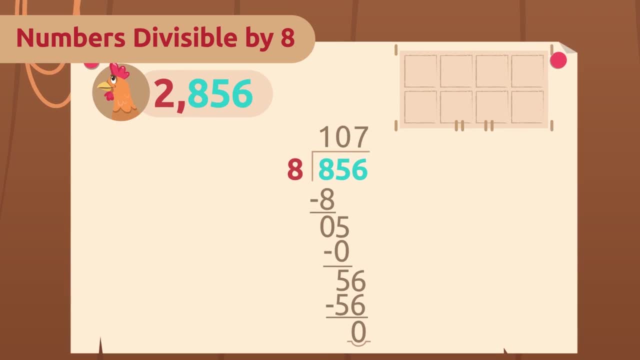 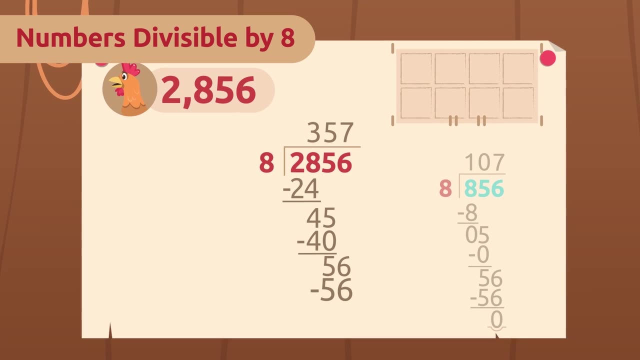 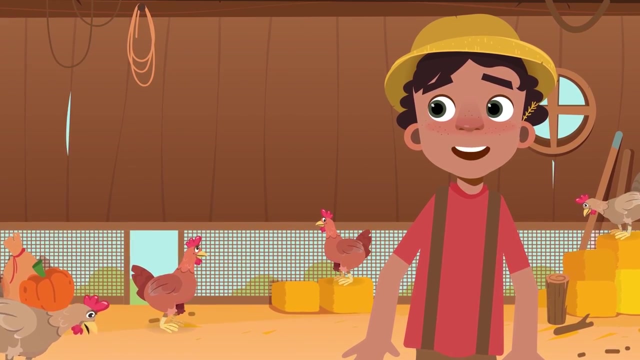 perfect division. This means that 2,000 856 is divisible by 8, and therefore no chicken coop will be incomplete. That's quite a few. I'll ask the whole Divisor family for help. Well, I'll start now. I. 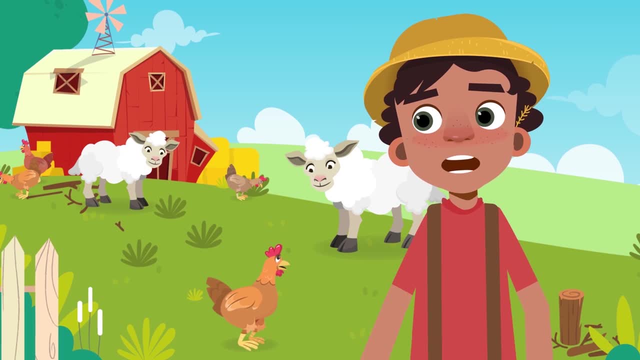 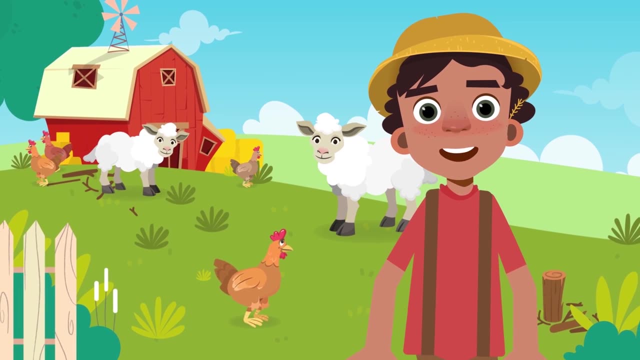 have a lot of work ahead of me and winter is coming. Why don't you stop by my family's restaurant? It's called Divisor Diners. My brother, Taylor, is the owner. I'm sure he'd love to meet you. He also uses some very curious 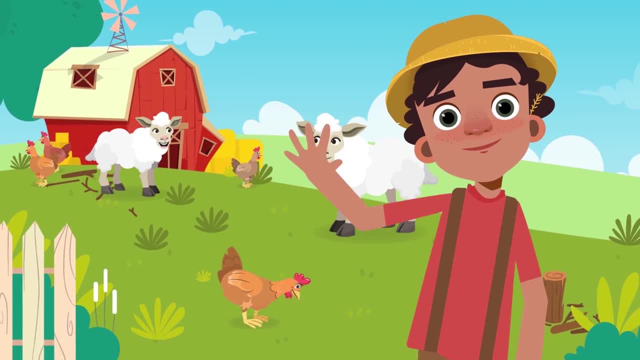 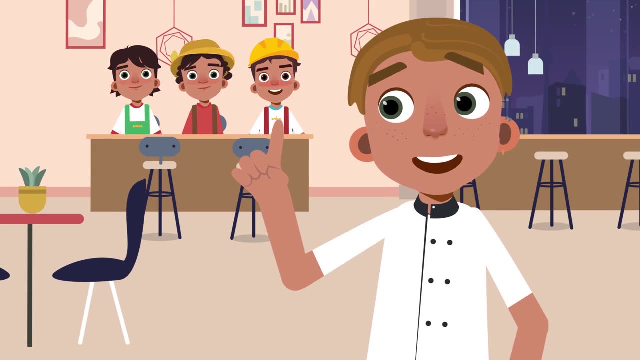 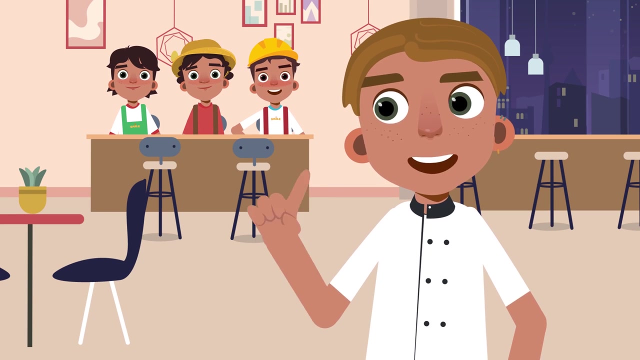 divisibility rules. You'll have a great time. Good evening. Welcome to Divisor Diner. Would you like a table for dinner? Oh hey, it's you who's been helping my brothers. I'm the oldest. My name is Taylor Divisor. I don't want to bother. 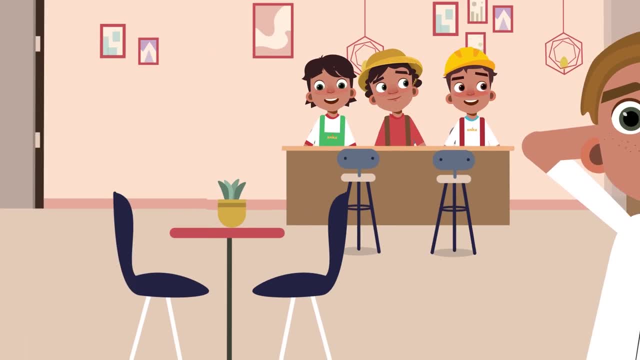 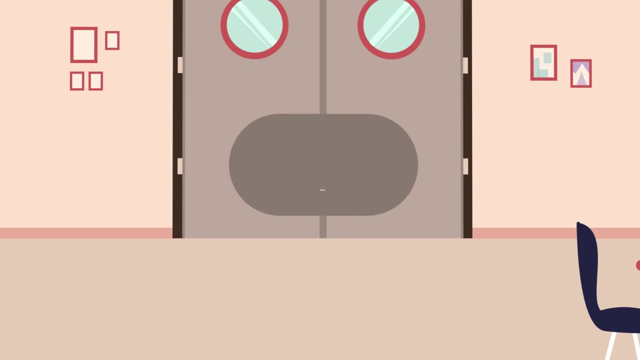 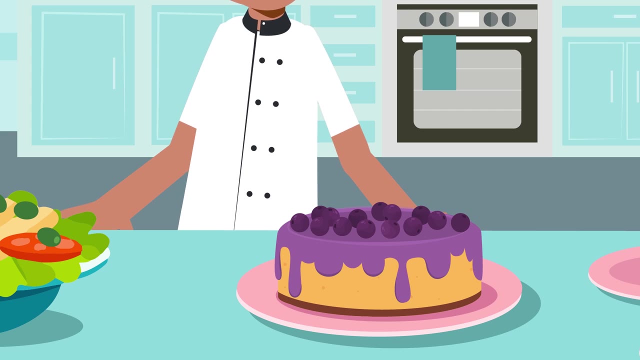 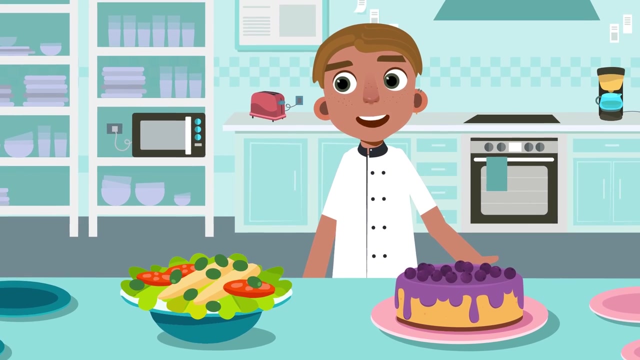 you, but could you give me a hand too? You can always watch TV. My customers love my olive salad and my famous blueberry tart, but I would like to know if any of the dishes will be missing ingredients. To find out, I will. 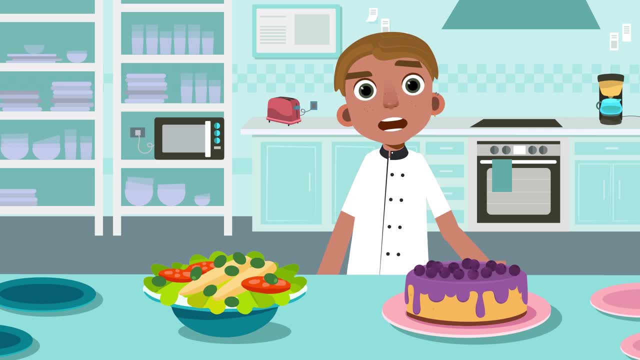 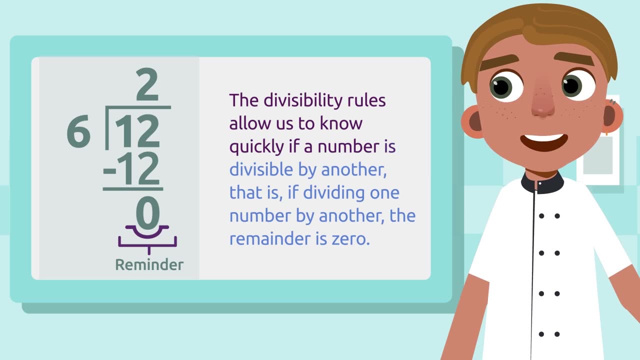 use the divisibility rule. Do you want me to remind you? The divisibility rules allow us to nice quickly if a number is divisible by another, That is, if this is differenceis divisible by a letter. How about if number 2? because this one is divisible? 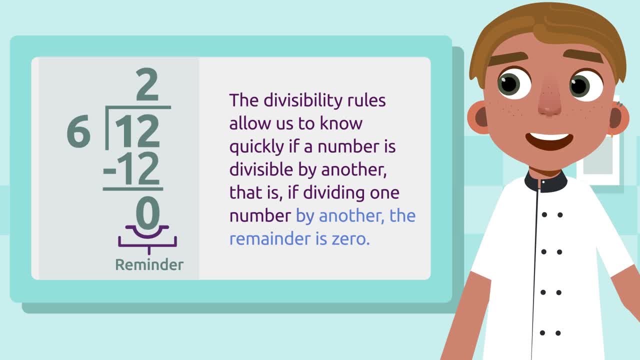 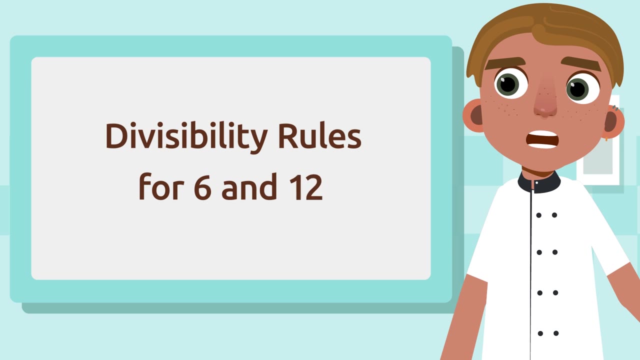 by another, That is, if, dividing one number by another, the remainder is zero. When a number is divisible by another number, the number that we have divided it by is known to be its divisor. Come on, I'll teach you the divisibility rules for 6 and 12.. 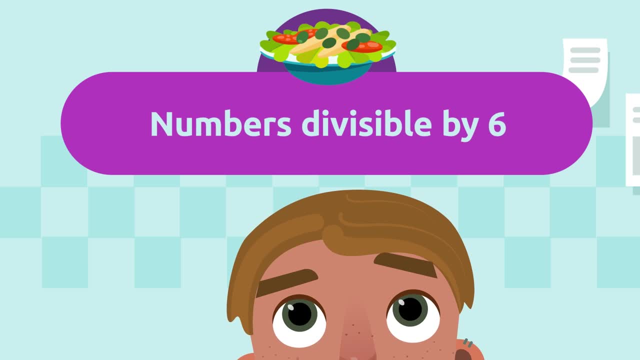 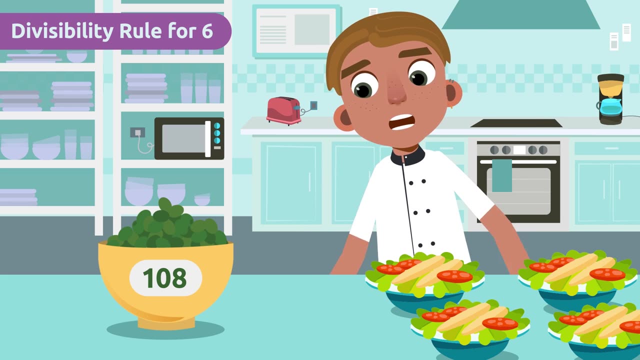 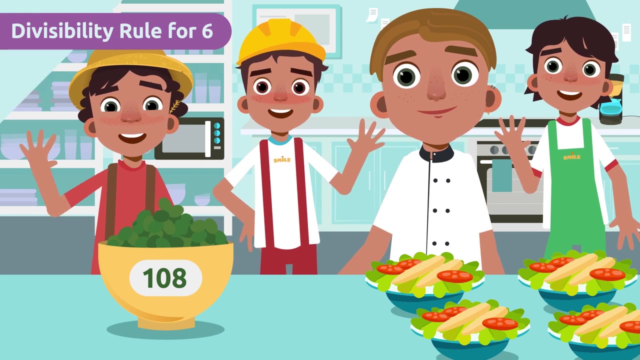 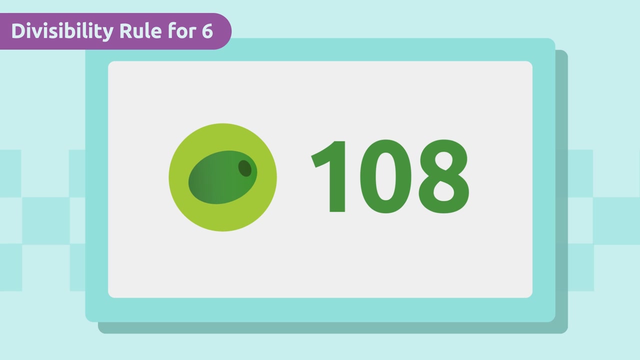 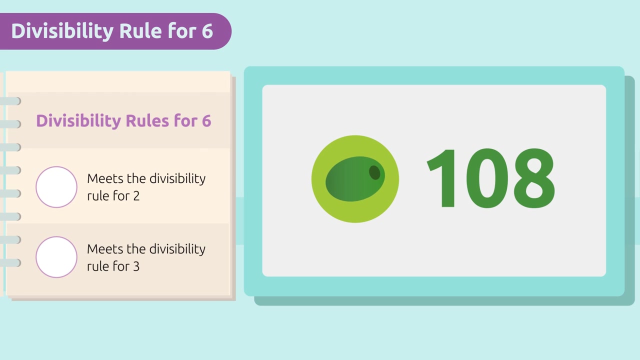 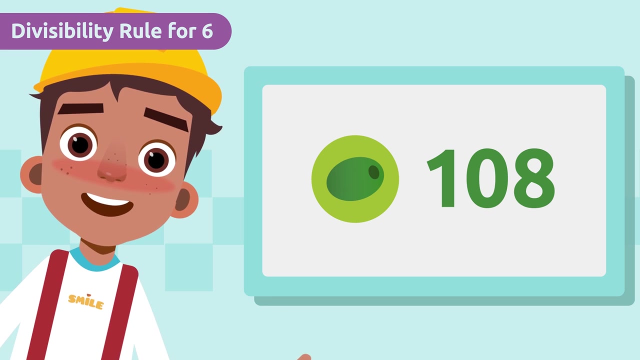 Numbers divisible by 6.. Numbers divisible by 6.. In 6, we have to check if it meets the divisibility rule of 2 and also 3.. Let's start with the rule of 2.. Windsor explained how to apply the divisibility rule of 2.. 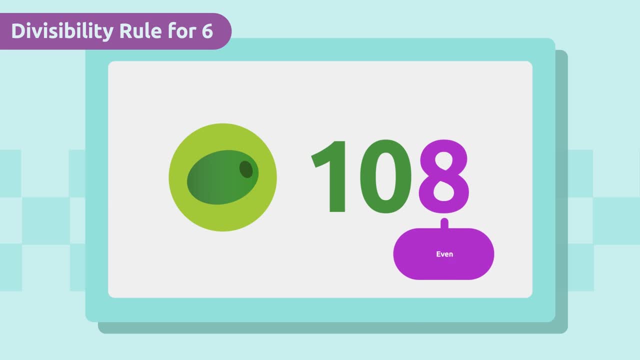 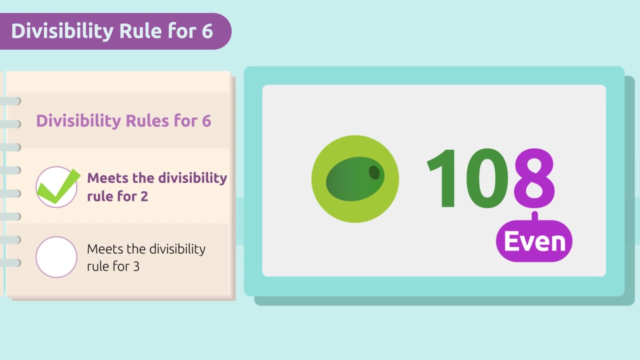 Remember we have to check if the last digit is even. Our number ends in 8,, which is an even number. so the rule of 2 is met. Now let's check the rule of 3.. Do you remember what Connor explained to you? 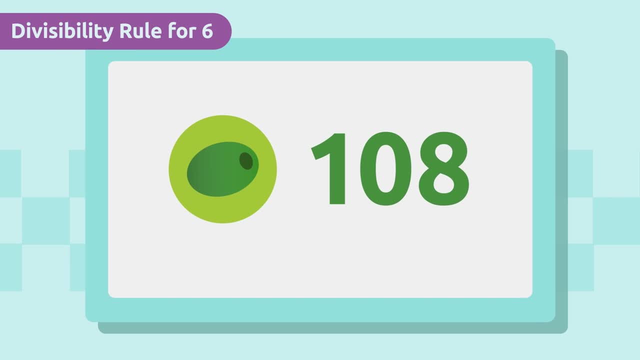 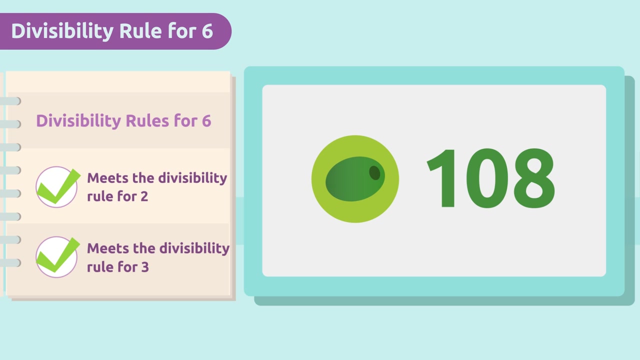 To find out if a number is divisible by 3,, first we have to add its digits. Our result is 9.. Since the number 9 is divisible by 3, the number 108 is also divisible by 3.. Now we know that 108 is divisible by 2 and also by 3.. 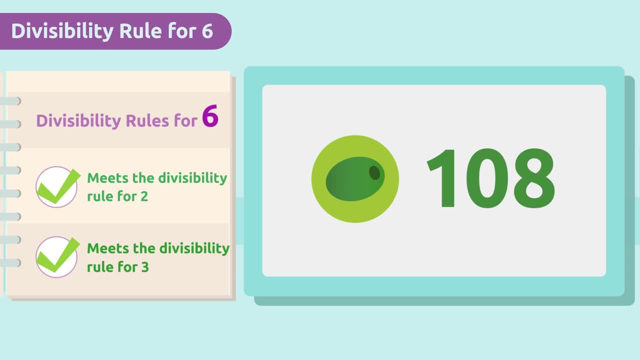 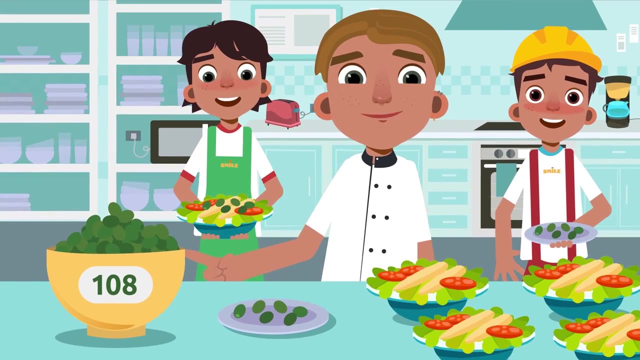 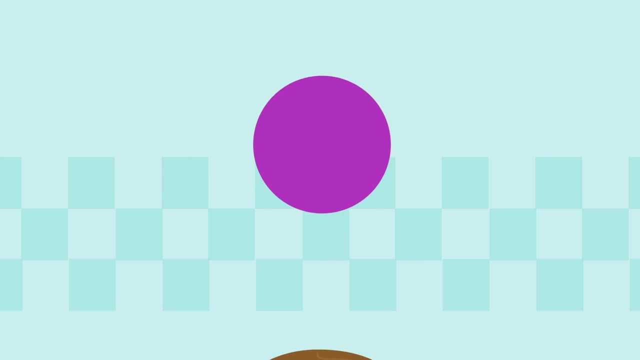 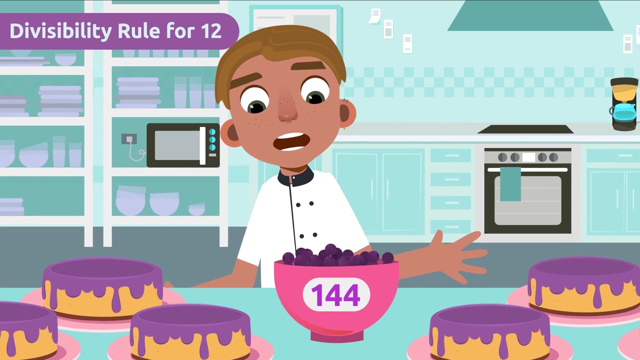 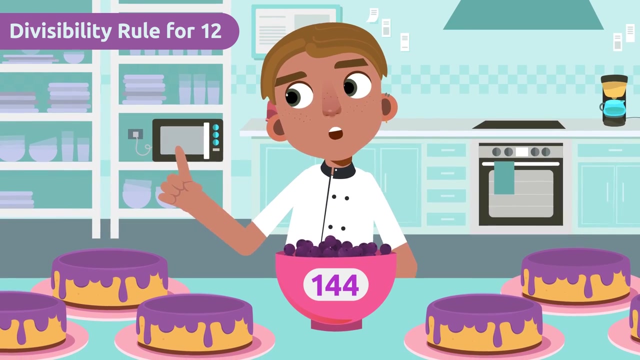 Numbers divisible by 12.. The restaurant's most famous dishes are 12 blueberry tart. There are 144 blueberries. The easiest way to know if a number is divisible by 12 is to check if it is divisible by 3 and also by 4.. 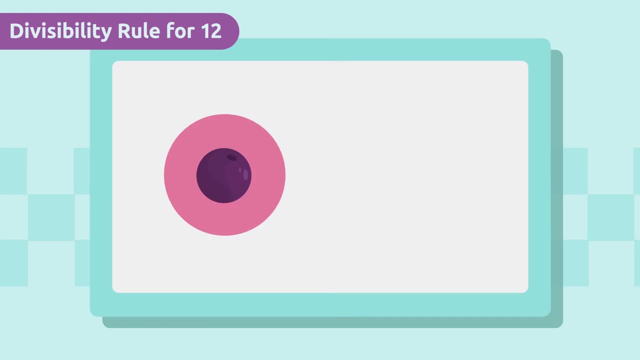 The easiest way to know if a number is divisible by 4 is to check if it is divisible by 5 and also by 6.. First let's apply the divisibility rule of 3, as we did before. Let's add the numbers. 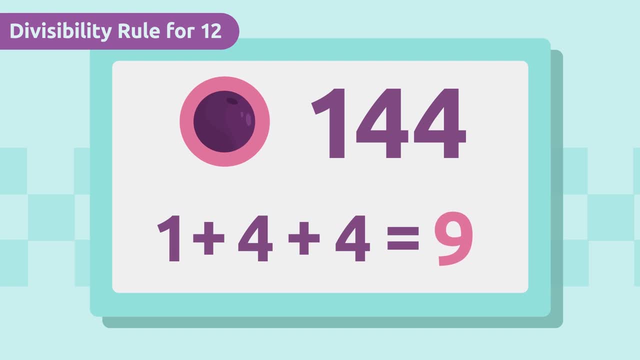 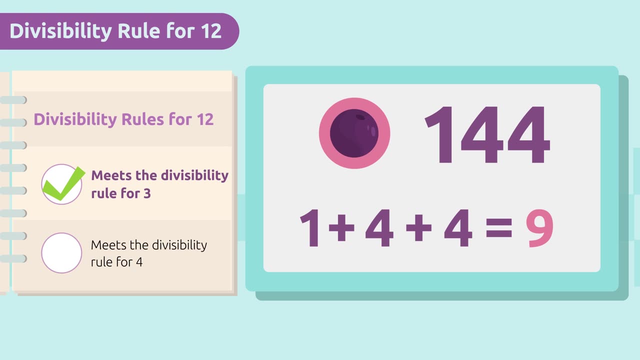 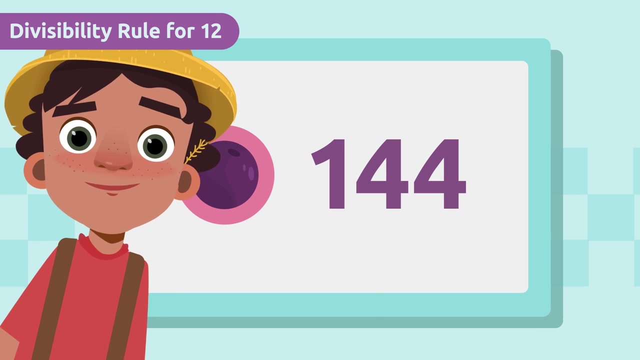 The result is 9. again, We know that 9 is divisible by 3, so 144 is divisible by 3.. Look at how quickly we figured it out. Now let's try the divisibility rule of 4.. As my brother Trevor, explained to you on his funnel video,